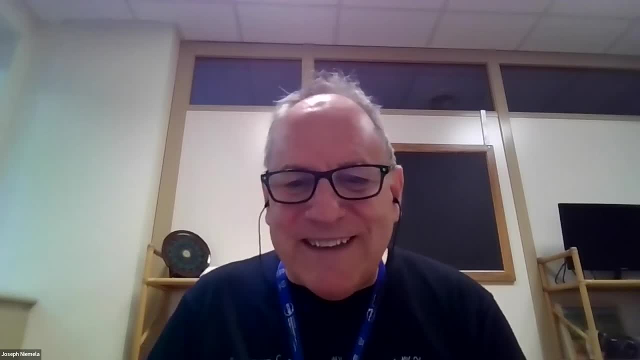 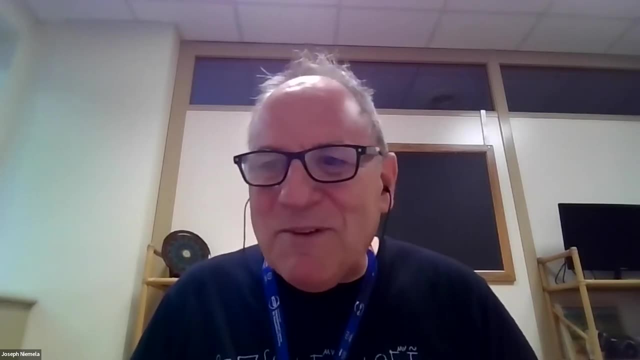 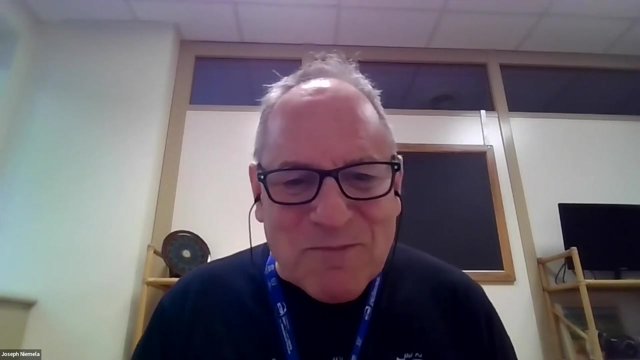 awards. actually He's got 81 papers, quite a few 18 patents. That's really great, Randy. So you can tell we're talking to technology people, But at any rate, so he's. I think you and Joe have known each other for quite some time. Oh yeah, we're peas in a pod here. 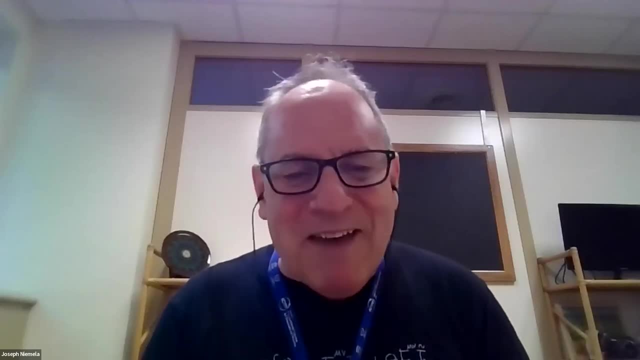 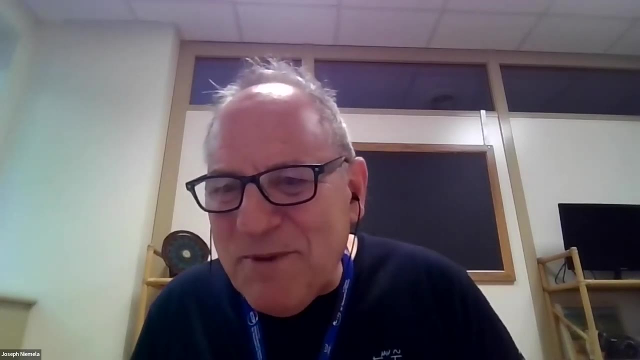 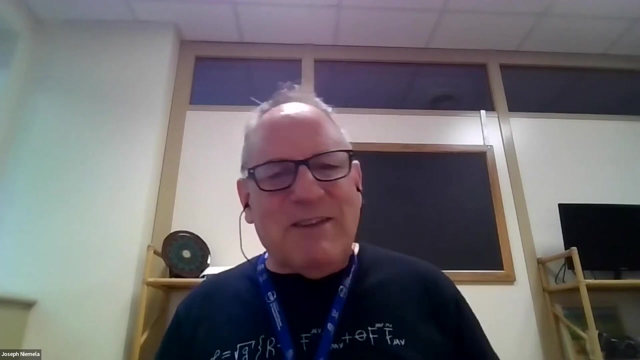 Peas in a pod. So, at any rate, we're really, really happy to have you come here. This is, by the way, I just want to let you know I've been. is John Howell Hooked up here? I don't see him. At any rate, I was talking to John Howell today And he was 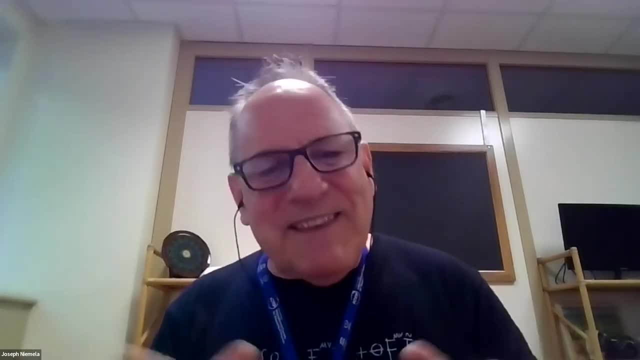 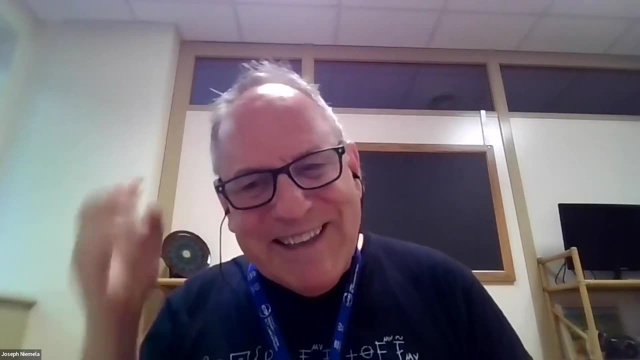 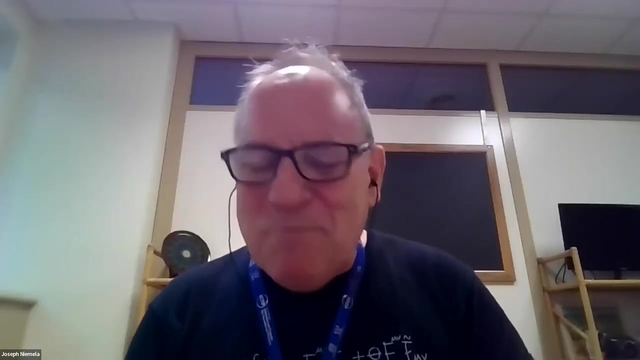 he was one of our speakers, lecturers yesterday And he liked this so much. We're thinking about making a program- you know, especially the thing with the honeybees- detecting landmines, Something, something kind of global, But at any rate. so maybe there's a spinoff coming out of. 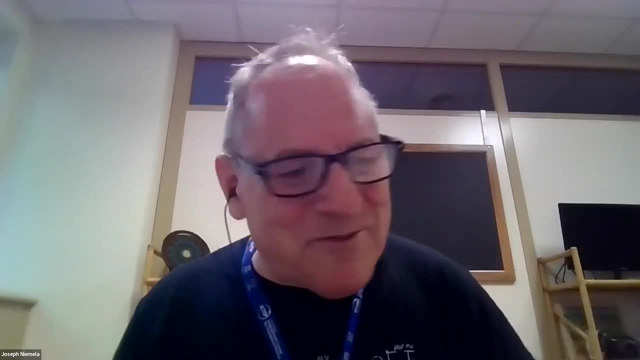 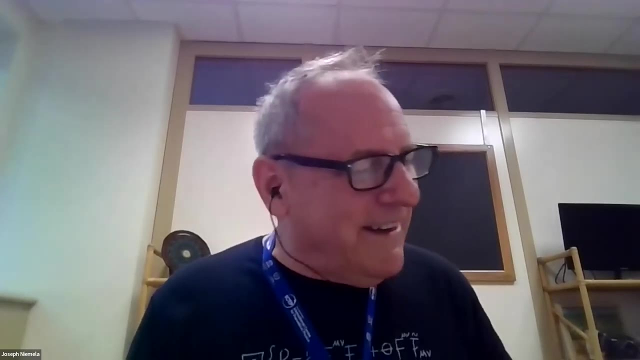 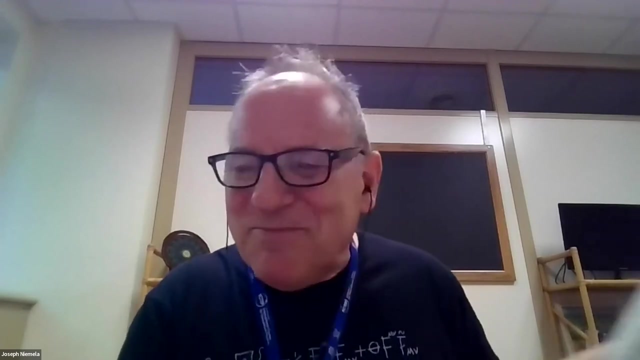 this Next year for the Day of Light celebrations. All right, So at any rate? well, Randy, I'll just let you go ahead and take over here. So you're going to talk about coherent LIDAR and digital holography. according to my schedule, That's the game plan. 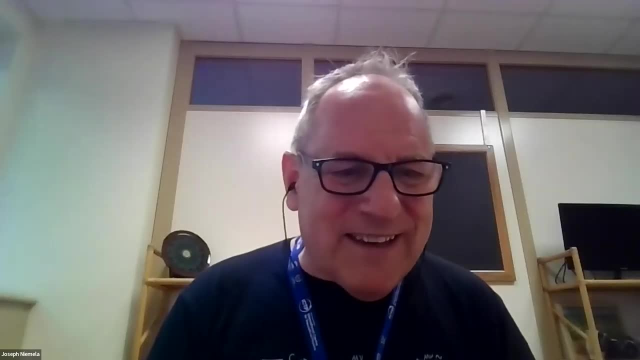 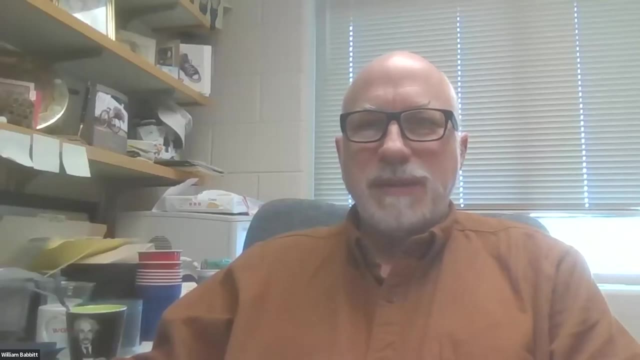 Let them know whether they can ask questions. They can raise their hand, Okay, No problem. Well, it's all up to you. Let me share screen here. Yeah, no problem, Just interrupting and asking questions And you guys can hear me. just fine, Is that correct? 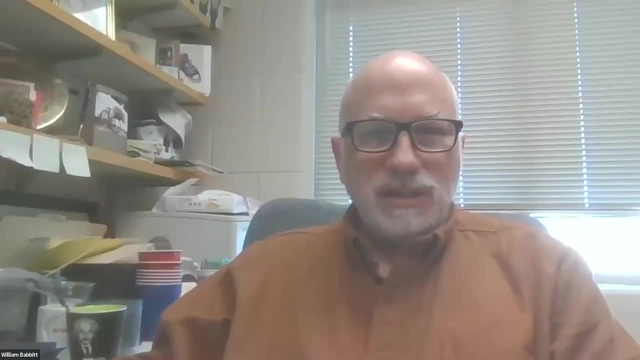 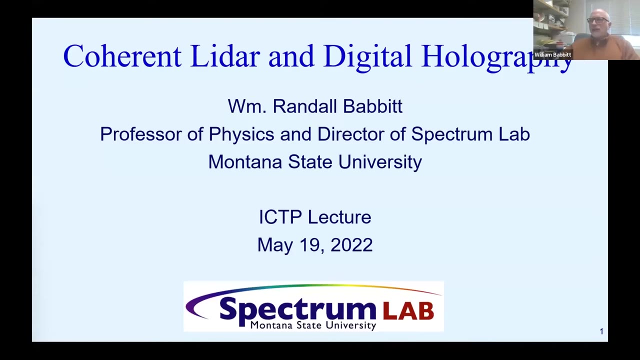 Yeah, All right, Let me get my screen shared. And which one do I want Screen two. There we go, All right, You see my Yeah, full screen. Okay, All right, And then pop that one up here, All right, Okay. 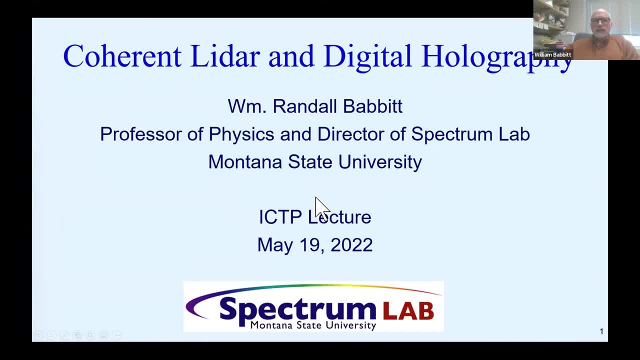 Hi, I'm Randy Babbitt And, as I said, you can hear me. I'm the host of Day of Light And if you'd like to interrupt me anytime with questions, um, uh, i guess abdul will monitor that. is that right and just uh. 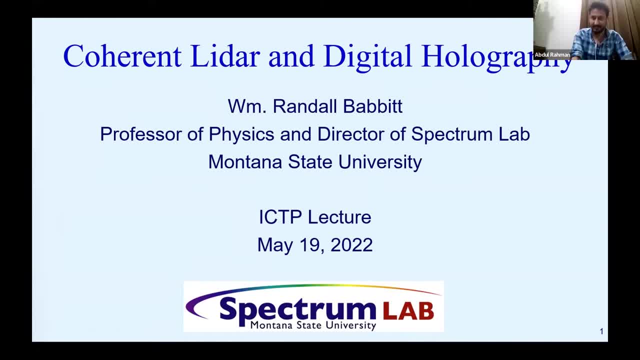 or someone will. yeah, yeah, abdul abdul will keep track of all those. okay, um, all right, um and uh. so i am a professor of physics, been here 25 years, and i'm director of spectrum lab, which i'll talk a little bit about the end, as well as a little bit about optec and montana optics companies. um. 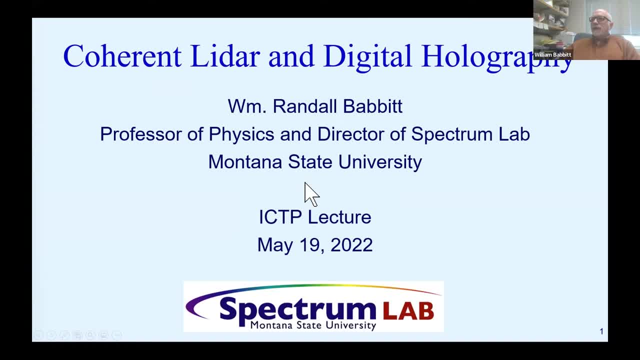 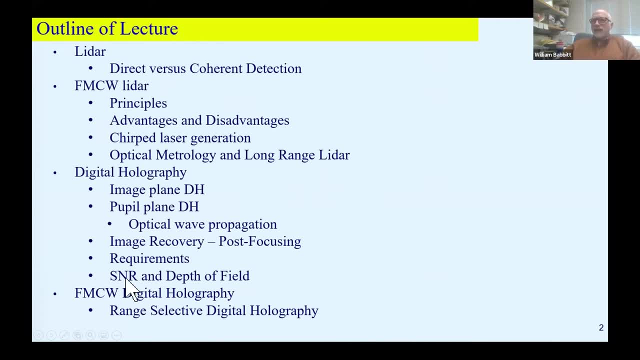 if we have time, um, and i'm going to talk today about coherent lidar and digital holography, which, um are kind of two distinct things, um, and in the end i'll bring it all together. um, so i'm going to talk a little bit about lidar, direct versus coherent, to begin with, and as far 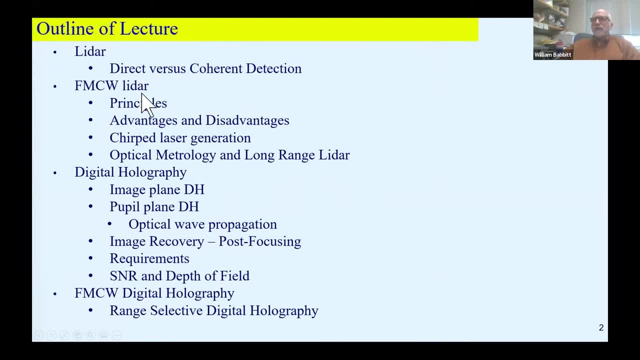 as uh coherent lidar. i'm going to really concentrate on fmcw frequency modulated continuous wave lidar, talking about the principles, advantages and disadvantages um chirp generation- which used to be a major problem but it's now uh second nature these days- and what it can be used for, everything from metrology of small objects to long range lidar. 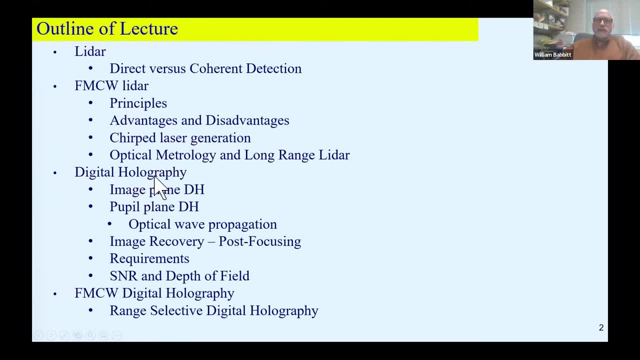 and then i'll talk about switch gears and talk about digital holography. um tutorial really on image playing, digitalography, pupil playing, um, when we talk about pupil playing, we need to learn a lot about optical wave propagation. so i'll go into that: how you get image recovery and how you can focus after the fact, after. 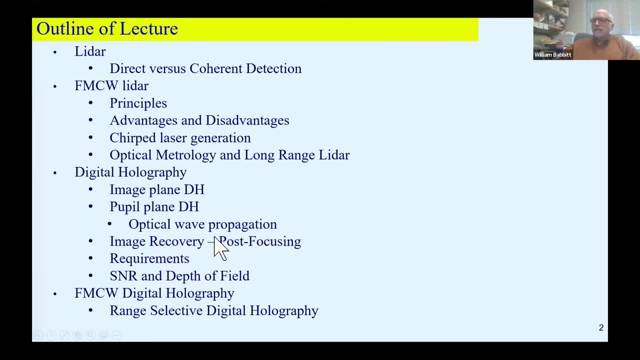 the recording, you can change your focus. in holography, um, some of the requirements, uh, the signal, noise ratios and depth of field you get with digital holography. and then i'll talk about fmcw digital holography, which is something we've developed here at montana state. uh, which is a 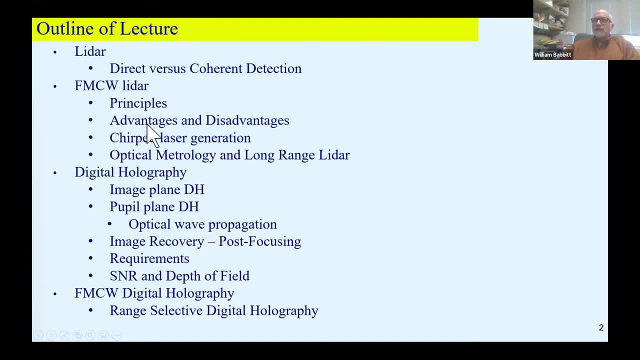 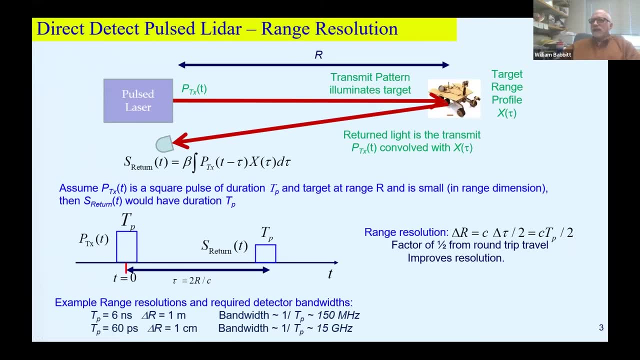 partnership between range selective digital holography, combining basically fmcw lidar with digital holography. so let's think about direct detection, lidar, talk about that and in general, what you do is you send out a pulse and we'll call it an intensity pulse going out. it's could be just a pulse. 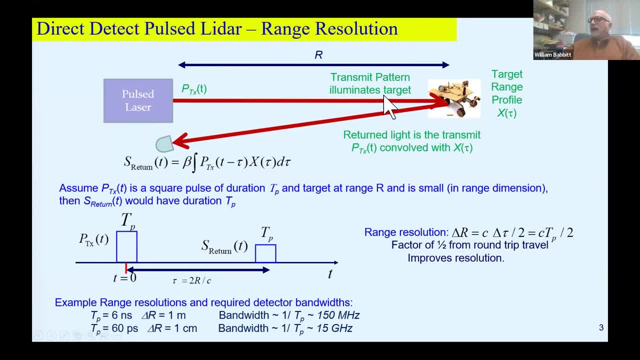 it could be a modulated pulse, but some something in time goes out, hits a target is actually a convolution of what you sent out with the target's range profile. So you get quite a convolved return here, a complicated return. But if you send a pulse out and the target is, 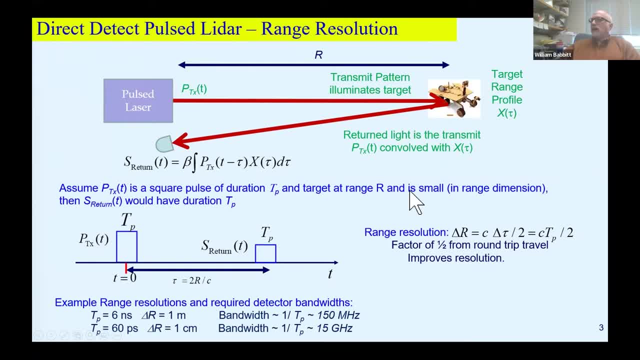 just some flat surface that is small with respect to the range, dimension. then you basically get a pulse back, And so we send out a pulse and we'll say that the pulse is only tp long. You wait a time, tau, which is basically the time it takes for the pulse to get from the transmitter to the 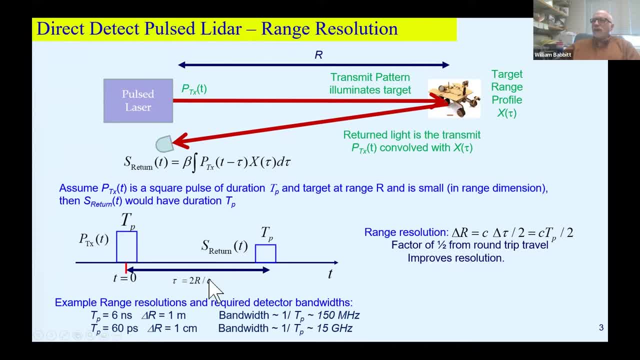 target to the receiver. So there's a 2r in there. divided by c, You'll get a pulse return, assuming your target roughly acts as a delta function. Your range resolution is just the derivative of this, So it's essentially your ability to measure. 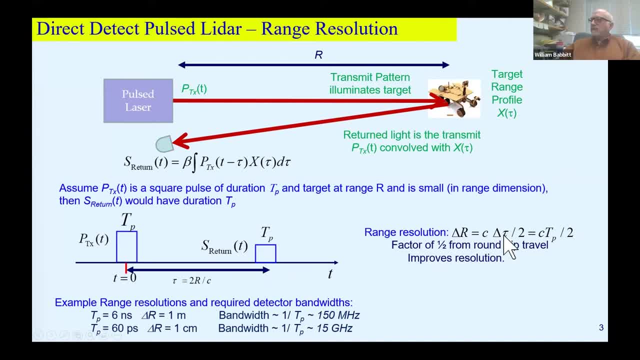 time accurately, And in this case that's roughly the width of the pulse. We'll talk a little bit about Rayleigh limit here in a second, why those two are related. And so if you have like a six nanosecond pulse you might get one meter resolution. You would need a detector that. could do that, And so if you have like a six nanosecond pulse, you might get one meter resolution. You would need a detector that could do that, And so if you have like a six nanosecond pulse, you might get one meter resolution. You would need a detector that could do greater than. 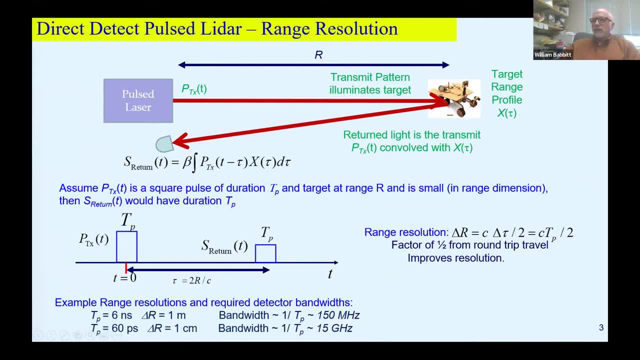 150 megahertz to see that If you wanted something more in the order of one centimeter resolution, you would need like 60 picosecond pulses or a 15 gigahertz detector, So pulsed LIDAR has an issue with range resolution requiring high bandwidths. 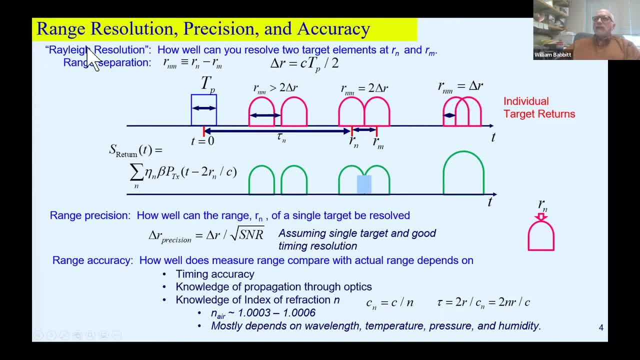 I just want to say a little bit about what you have about range resolution. There really is range resolution, precision and accuracy And you have to keep those apart. Resolution is really your ability to resolve and it's really related to spectro. 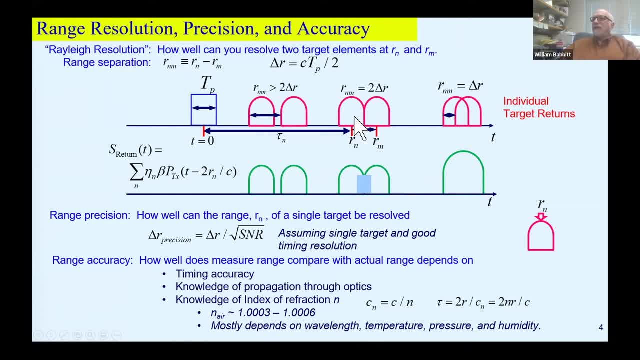 Rayleigh resolution. It's when two targets can be resolved and aren't on top of each other. And here I'm showing three cases. one, where two targets are well separated, greater than their range resolution, twice the range resolution when they're separated by twice the range resolution. 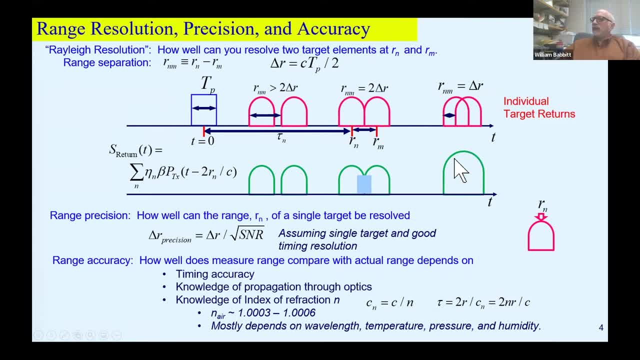 and when they just become really just one block of the piece. It's a little bit of a thing, but it's blob is when they are one range resolution. So here are the separated individual target returns And then if you combine those we can see that when you get down to the separation 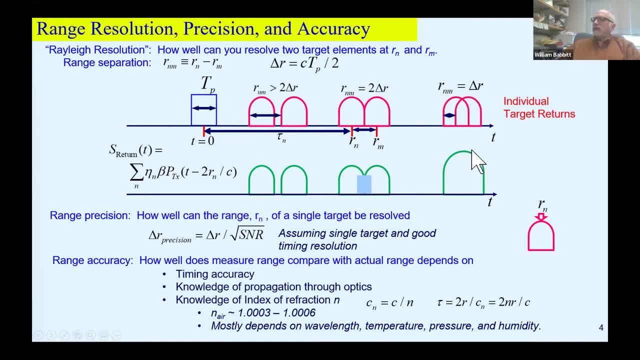 being between the two, targets being the range resolution, you just looks like one blob and then you lose their individual characteristics. So that's your range resolution And in essence that's the basic. the pulse width times C divided by two. Your precision can be much greater, though. 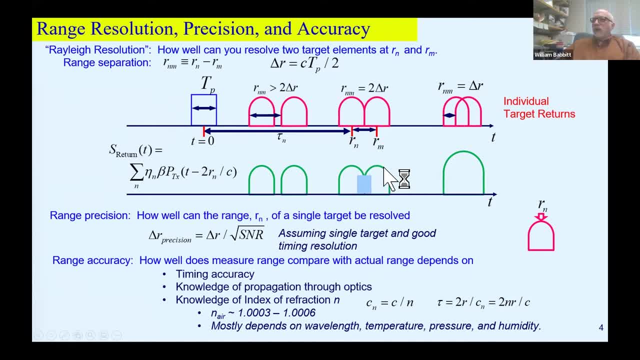 because if you only have one pulse and you wanna know how precisely you can identify where that target is. if you've got good SNR, you can basically find the center of that blob to basically the range resolution divided by the square root of the signal to noise ratio. 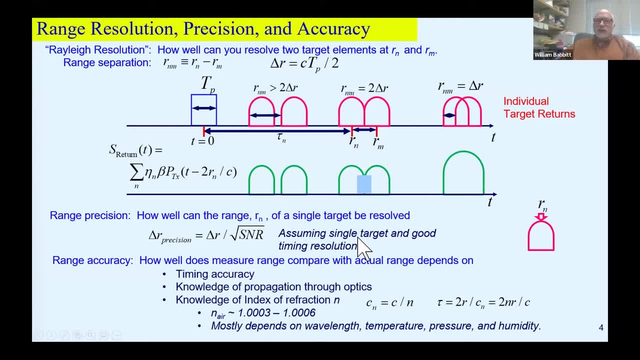 And so you can zero in on the center. It does assume you only have a single target and he had some good timing resolution. but you can get good signal in noise. You can get much better precision than you have range resolution. And then accuracy is another thing. 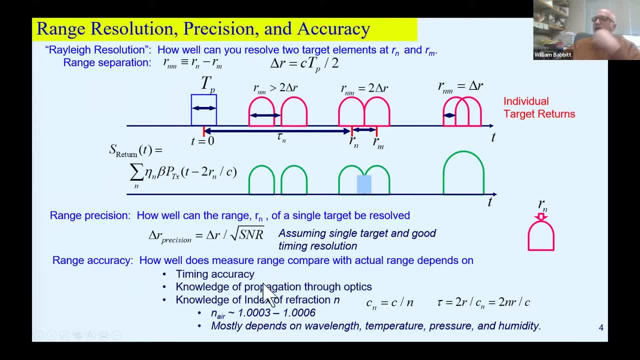 That depends a lot on has many things that. it depends on your timing, accuracy, your knowledge of the propagation through any of the optics as well as the atmosphere, or wherever you got what you're going through, the index or refraction. 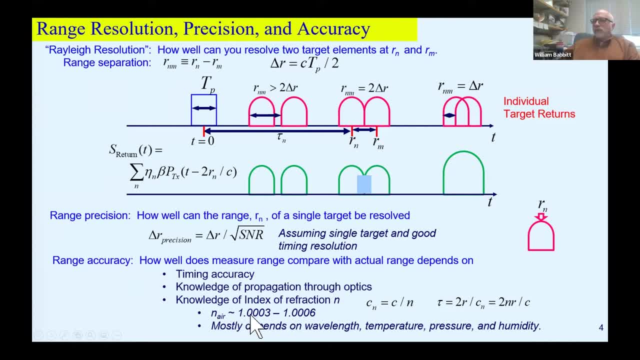 the difference between assuming error is one or two miles, midway through solar eclipse and it's actually, and the air is 1.0003 or 0006, depending on where you are, what your temperature, wavelength, pressure and humidity are. you can get considerable errors If you are a kilometer out. 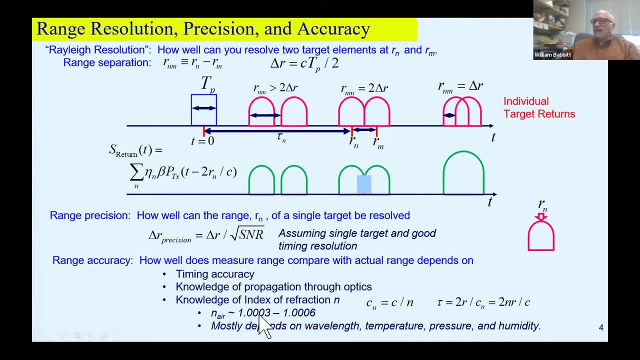 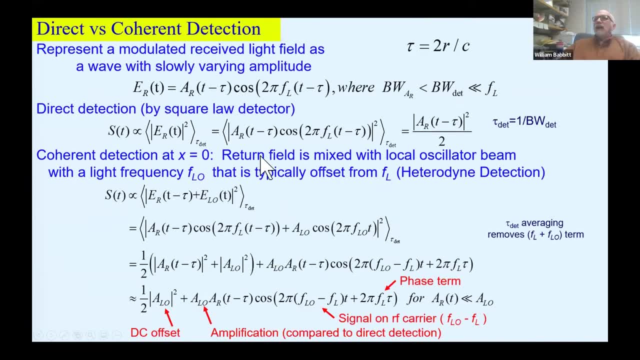 this is on the order of 0.3 meter error if you assume the wrong index. Now let's talk a little bit about direct versus coherent detection. Here is a light field with an amplitude. It's light field returning from a target, so you have an amplitude that's delayed. 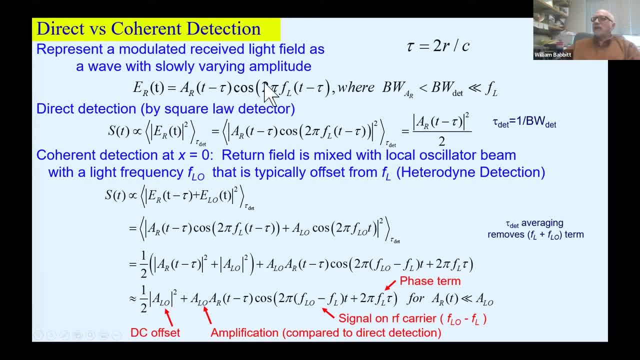 by the round trip to the target. It's on a cosine background, a sinusoidal background, also delayed with 1.0003.. The assumption here is that we can detect the intensity of this pulse, so the bandwidth of your modulation this pulse is less than the bandwidth of your detector, which is much less. 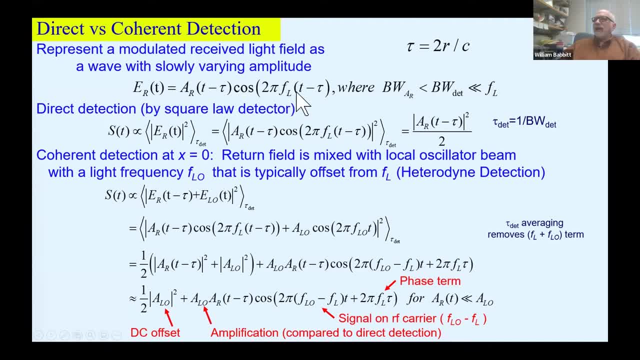 than the wavelength of light or the frequency of light. So you can't detect the frequency of the light, but you can look at the intensity of this In direct detection. that's what you do. A detector is really a square law detector. 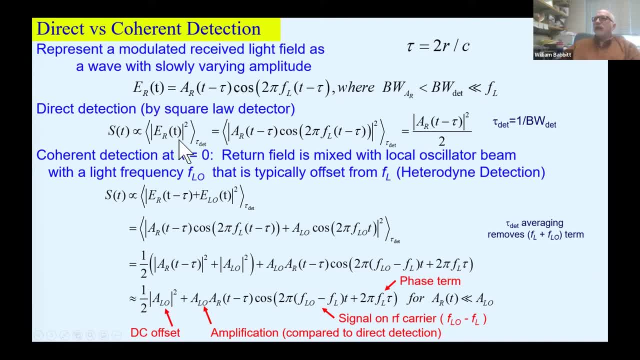 And what that does is it squares your optical field and then averages over the integration time of the detector, which is roughly one of the bandwidth of the detector. And so if you take this and you square it and then average it, you lose. If you square a cosine, you get a DC term plus something that's beating at twice the. 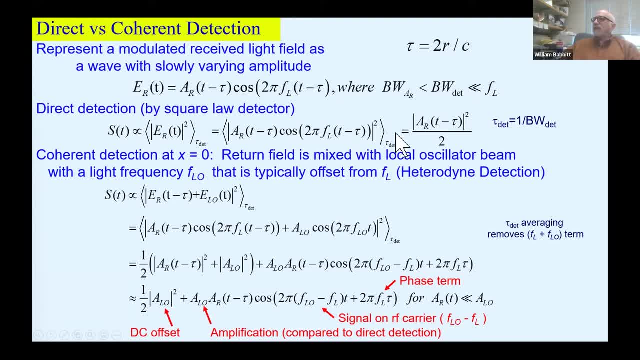 optical frequency. The averaging gets rid of that twice optical frequency and all you see is the envelope squared. when you do direct detection, When you're doing coherent detection you will mix the optical field with a local oscillator. So we'll take the delayed return signal. 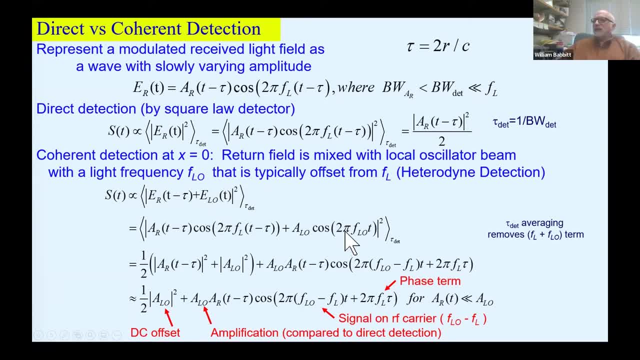 and mix it with a local oscillator, which you define as a cosine, But typically we do this at a different frequency. It's heterodyne detection rather than the homodyne detection. So we mix the return signal which is at frequency of the late. 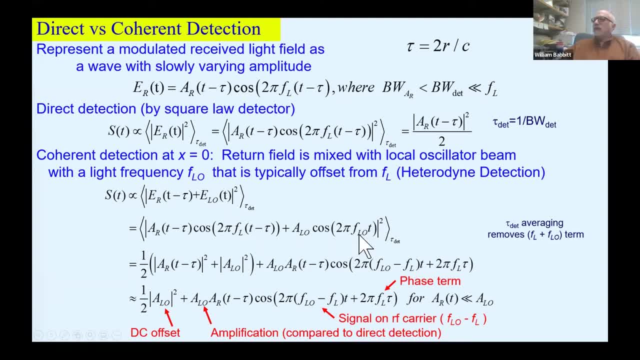 with a different transmit laser, with a different laser that is slightly shifted, And we look at the intensity of the combined signal. If you look at the intensity of the combined signal, you have the intensity of the pulse that comes back, You have the intensity of 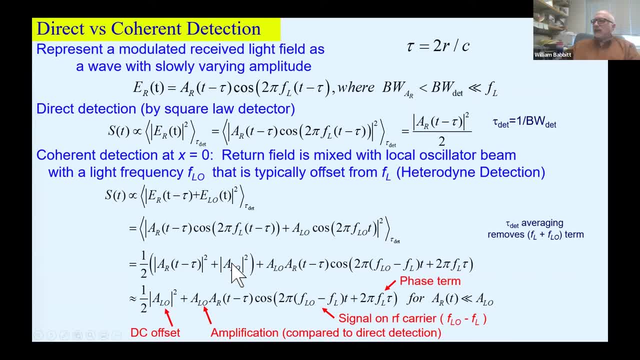 the local oscillator, which is flat in amplitude, And then you have the combined term. here the FLO plus F laser term gets averaged out. so you only have the difference frequency. So you get a signal back with a beat on it that has an amplitude or an envelope. that was the envelope. 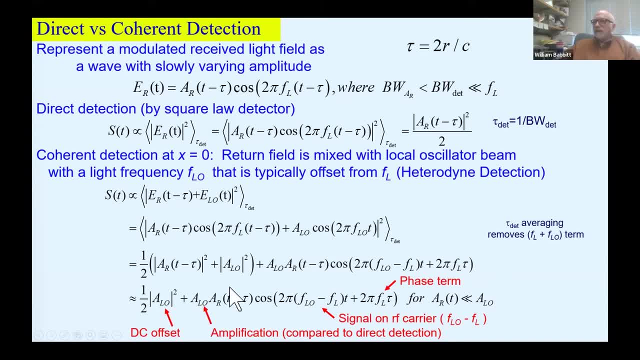 of the return pulse, And if your LO was much greater than your return- which is what you want when you're doing coherent detection- then you can ignore this term here and you basically have an optical carrier, which is nice because it's removed from DC, making it a nice DC offset. 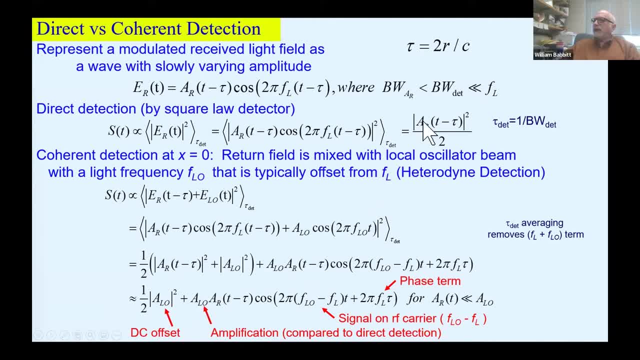 You have an amplification here of the return signal. Up here you had AR squared, Here you have ALO AR, So you really get an amplification of the ratio of the amplitude of the LO signal divided by the amplitude of the return signal. It's on an optical carrier, which is nice because it's removed from DC, making it a nice DC offset. 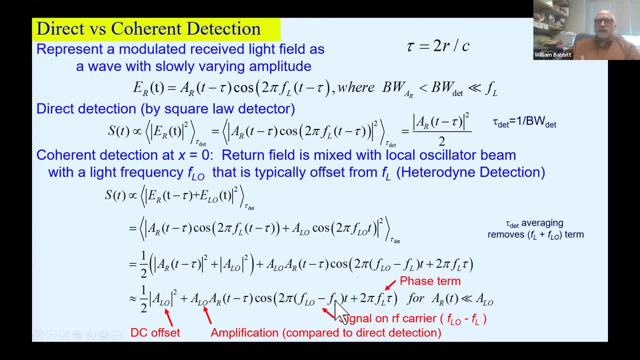 It's a little easier to detect and you can adjust this frequency so that it matches whatever detector you're using. And there's a phase term here which usually we ignore. but it's actually interesting because one, if there's actually added phase, that can destroy your signal. But you can. 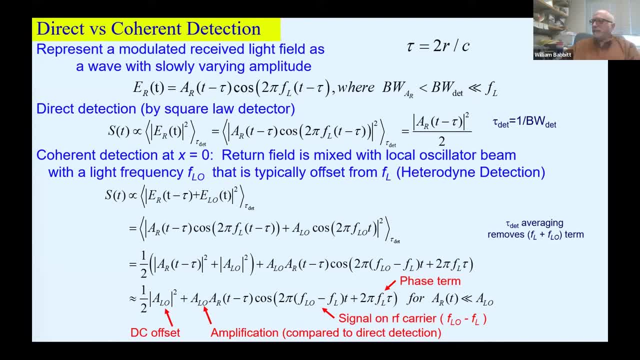 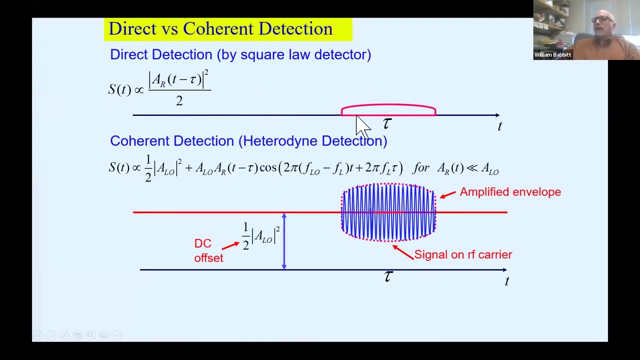 actually use this to do things like frequency shift of holography or study vibrations or Dobler movement of a target. This phase term can come in useful in many cases. So pictorially, here we have that, this direct detection. you basically just have a blob coming. 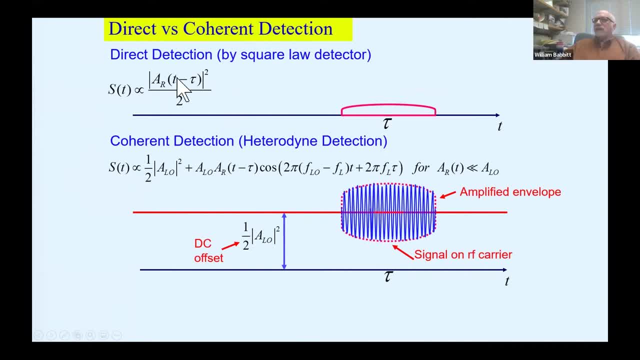 back with the envelope squared of your return pulse And the coherent detection. you still have the envelope, but it's modulating a cosine and riding on a DC background. So this is just a pictorial way of looking at what we were just showing before. 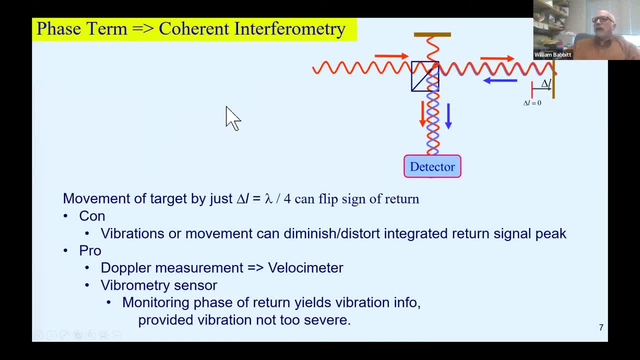 So the one issue with that phase term is that if something is moving, if your target's moving on the order of lambda, that can switch that cosine from. if you go lambda over four, switch the cosine from a sine to a cosine, which can be a problem because 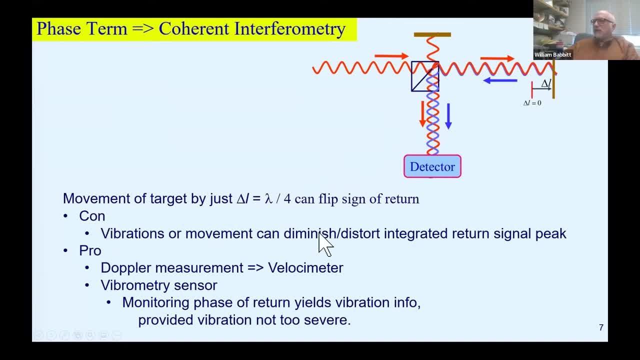 vibrations or movement can really distort your signal or diminish your return if you integrate it. But, like I said, the nice thing about that is that that phase term can also give you Dobler measurements symmetry. If the movements are small, you can actually study the vibrations of a target. 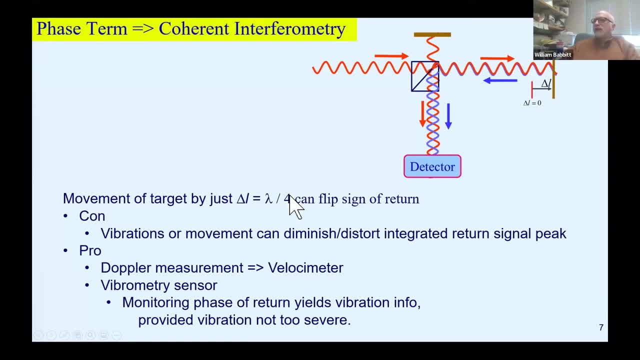 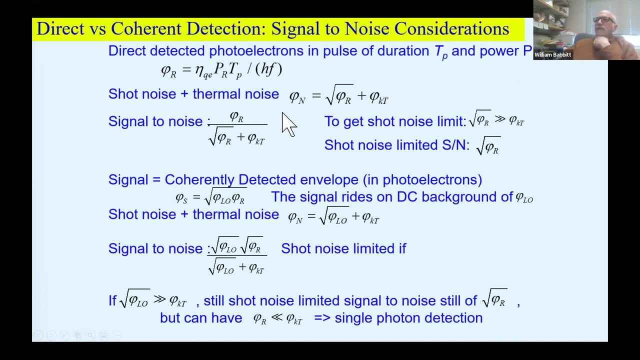 through that phase term, But I'm not going to get too much into that, I just wanted to mention that. So the signal-to-noise considerations: If you have direct detection, then your signal-to-noise is basically governed by the power of the return, the duration of the pulse that comes back, your quantum efficiency. 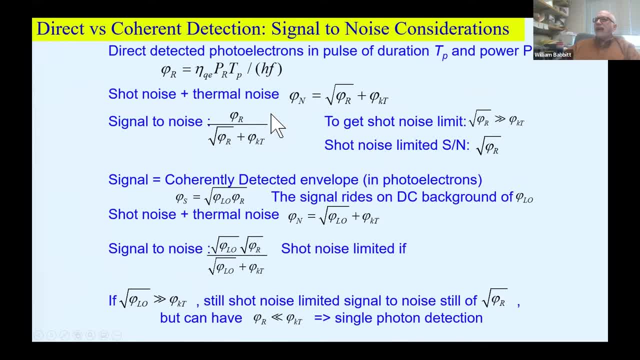 Planck's constant and the frequency of the light. The noise is usually the simplest way to look at it. It's the shot noise, the square root of the return photons, plus thermal noise that's in band, And so your signal-to-noise would be the ratio. 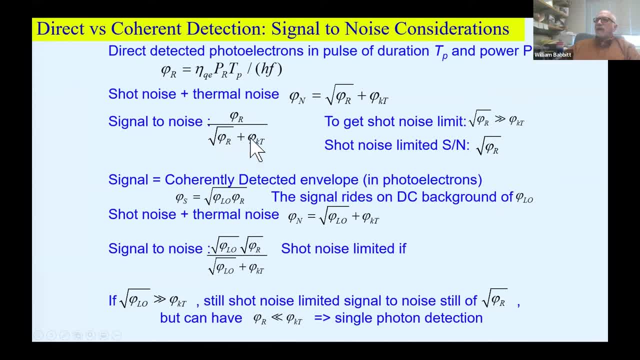 of the number of photons that get back square root of number of photons plus photons and the photoelectrons. actually in photoelectrons and the thermal noise. in order to get to the shot noise limited you need to have your number of photons in your signal much. 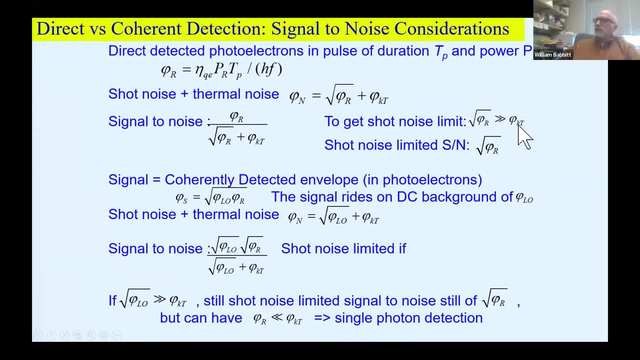 greater square root of that, much greater than the thermal noise. so you have to have very strong signals to cut back in order to be shot noise limited when you're doing coherent detection. your signal is the square root of the number of LO photons times the number of return photons. your noise is the square. 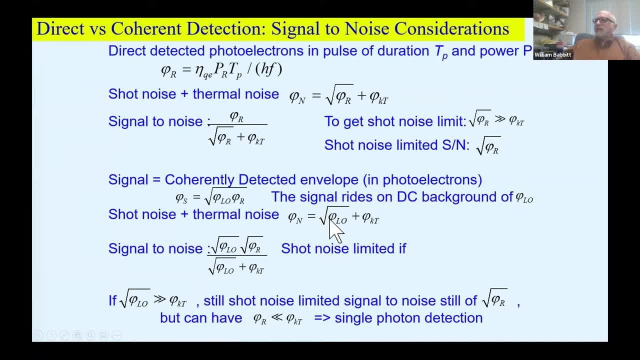 root of the local oscillator which dominates. it's actually the square root local oscillator plus Phi R, but we usually ignore that part, plus the thermal noise. if you look at your signals and noise, rather than the number of photoelectrons and the return, it's the square root of the number of photons. 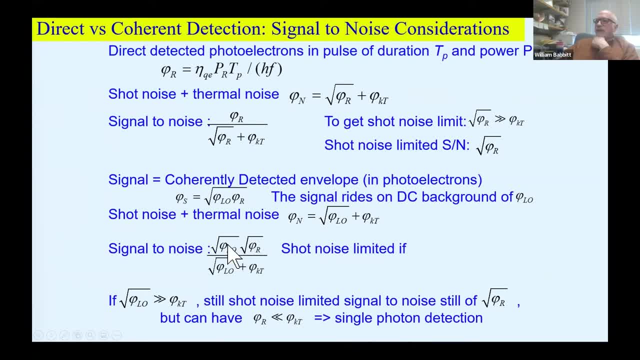 and return times: the square root of the LO. the interesting thing about this is, if you have a really strong LO, then these two terms cancel out. this is much greater than this. you can actually get to a shot: noise- limited detection. square root of the number of photophoton. 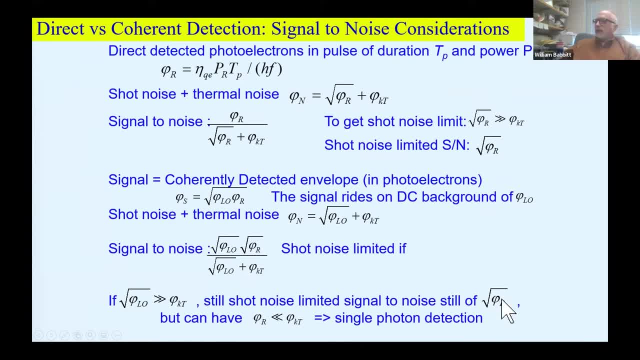 electrons in the return, and you can do that in a case where the number of electrons- photoelectrons- is much less than the thermal photoelectrons. so you can actually know what comes out if you run it from two levels. notice: the two levels of título is not as noticeable. 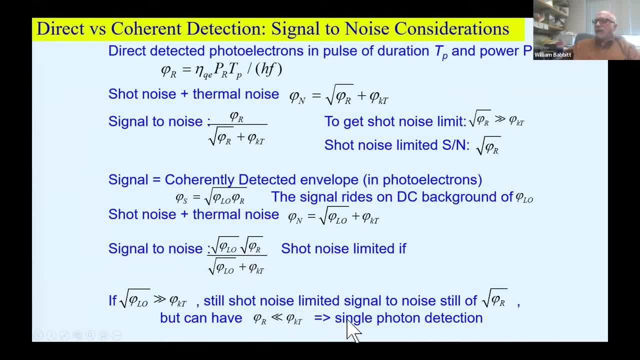 so you can actually look at the counter and you can say, okay, so in the against spots on the chiffon rows, that change too. can you ever test your can actually get single photon detection even well, even when you have thermal noise, well, the thermal noise. so that's one nice thing about coherent detection. 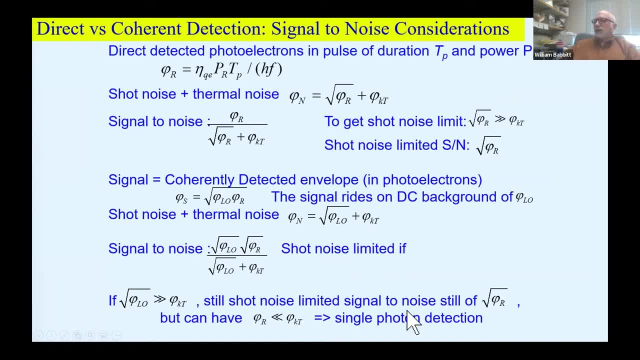 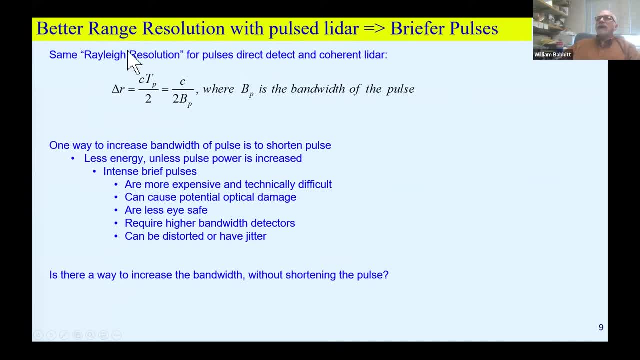 is that you get that amplification to the point where you can actually get signal to know, shot, noise, limited signal detection. let's talk about the, the what it, what it takes to get good resolution with the pulse lidar. like we said, the range resolution is a function of the duration of the pulse, which is also 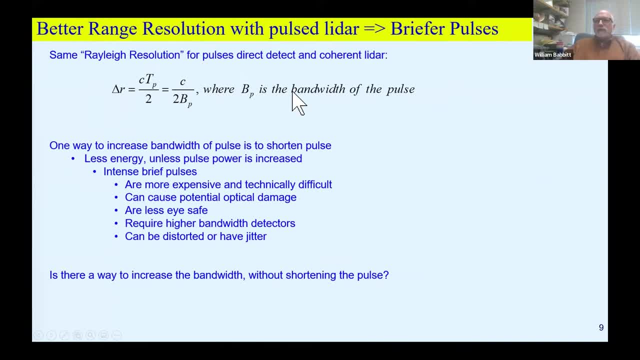 inversely related to the bandwidth of the pulse or the bandwidth detector. you need to measure the pulse, so one way to increase your resolution is to increase the bandwidth or shorten your pulse. if you don't increase your power, that's less energy. so usually in order to get 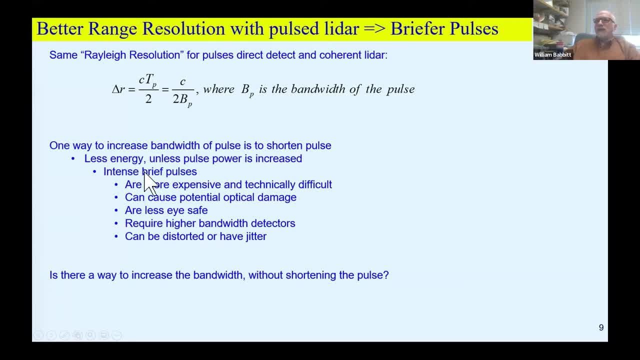 a keep your signal noise the same, you have to have an intense brief pulses that can get expensive and technically difficult. brief optical pulses can cause optical damage. they can be less I safe. they require high bandwidth detectors to see them and there can be distortions and jitter in the creation of those pulses. 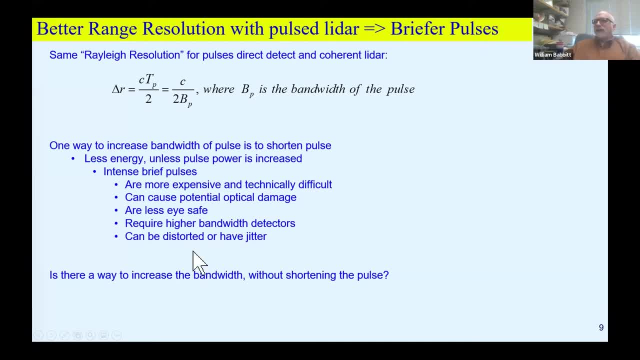 so that's why we go to FMCW, because it doesn't require shortening the pulse. it's a way of increasing the frequency of the pulse. so that's why we go to FMCW, because it doesn't require shortening the pulse. it's a way of 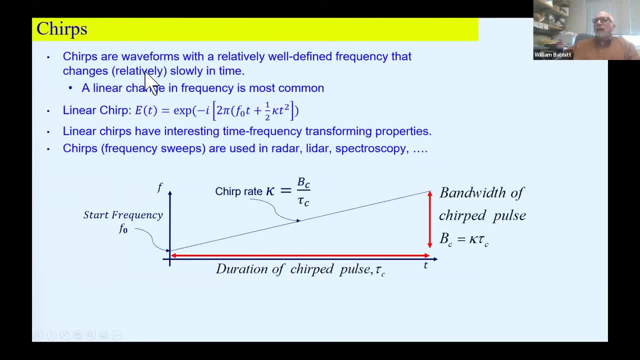 increasing bandwidth without shortening the pulses. so FMCW is based on chirps, chirped pulses. what's a chirped pulse actually? I think Joe should do this. he did a really good sound of chirps the other day, but I'll try it. our chirp is, but listen to Joe's, but he's better, better recording. so what is? 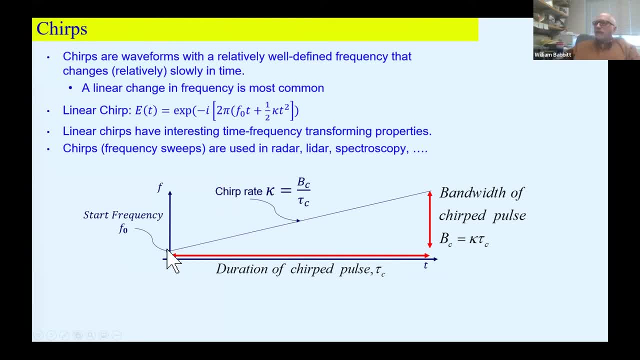 a chirped pulse. a chirped pulse is a pulse that starts at one frequency and ends up at a different frequency and literally ramps from that starting frequency to the end frequency over a certain bandwidth, bandwidth of the chirp- and it does let over a duration- tau C, and you'll see these bandwidth chirp. 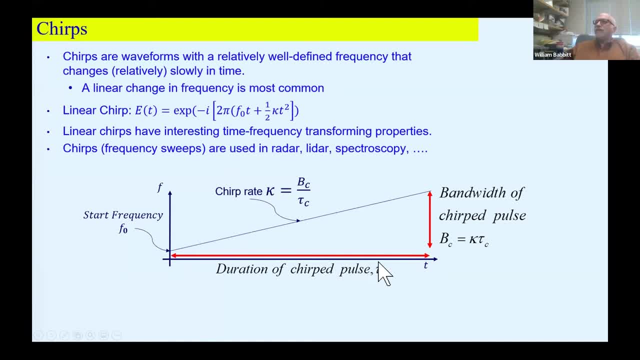 duration of chirp a lot of times. so remember those at a chirp rate, which is the ratio of the bandwidth to the duration, and you'll see that a lot too. and mathematically you can write that as here, where we see, there's this one half Kappa tau squared because the frequency is the. 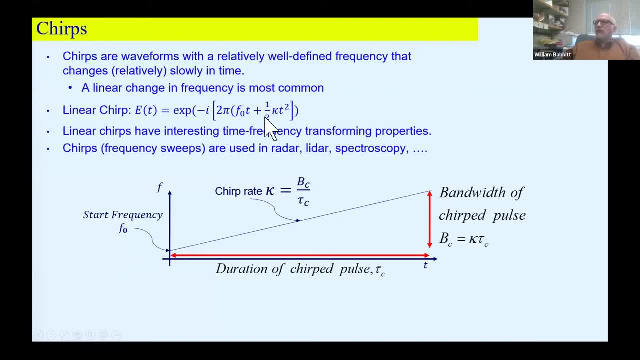 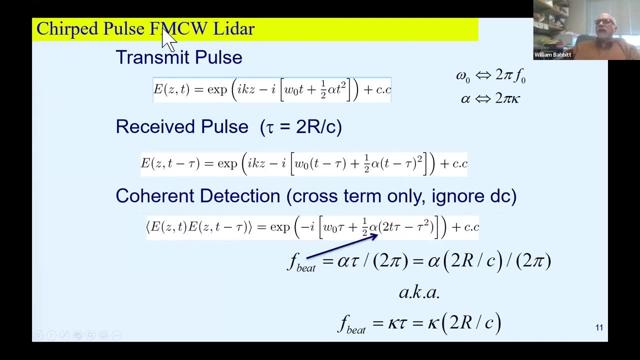 derivative of this phase term. and so if you look at the frequency, at the frequency F naught, the derivative, this would be F naught plus Kappa T, and this is the phase here of the linear chirp. all right, so let's look at what FMCW. 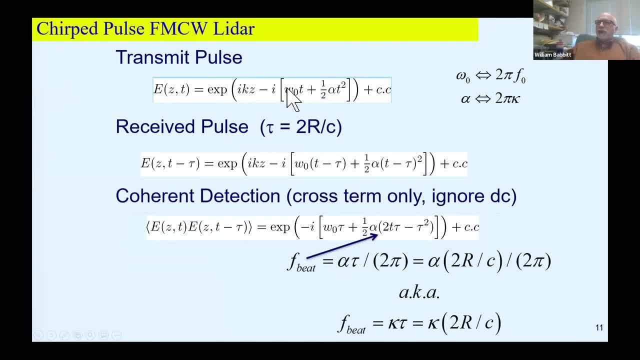 LIDAR how it uses that. if you send out a transmit pulse that mathematically looks like this, which is, by the way, I've converted to angular units here, so so you have the frequency of the laser times time and one half times the chirp rate converted. 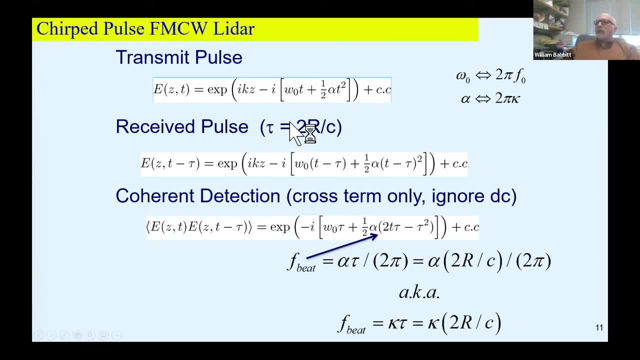 with two pi Tau T squared, the received pulse comes back tau later. so it's the same equation: we're just with T minus Tau's in it. and then, when you do the coherent detection, you beat those two together, which really is really just a contraction of these two phase terms, is what you end up with. and if you look at, 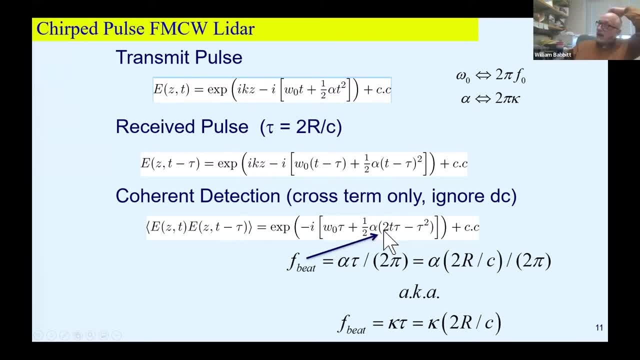 that what's left over when you beat those two together and get rid of the high frequency terms. you spatially filter it or look at the intensity averaged a little bit. there'll be a term that there will be a phase term. that's a function of the frequency of light, but there's this term here which is very 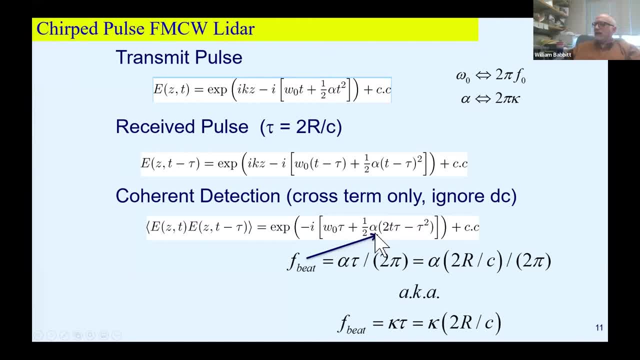 interesting. the two is cancel and you get alpha T, tau, or in terms of Kappa's Kappa Tau, which is a beat frequency, and that beat frequency, Kappa Tau, Tau, was related to the range. so you at this beat that is proportional to the range. so if you measure this beat frequency of the coherent detection and 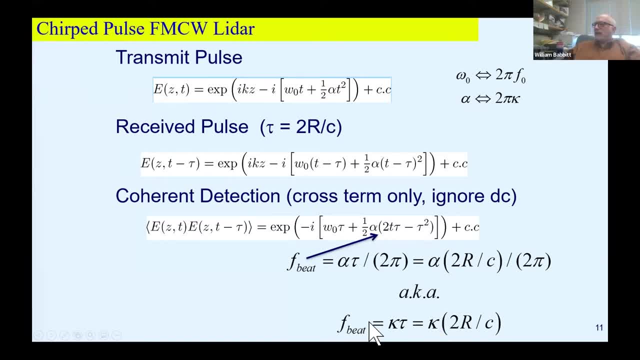 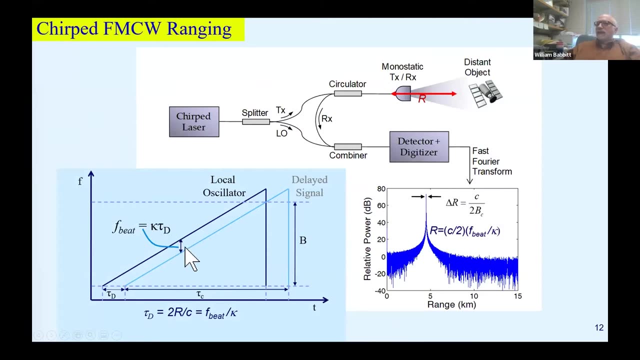 you basically divide it by Kappa and multiply times C and divide it by two, you will get the range. so that's how you basically convert FMCW signals. you take a, take a- let's switch over here. you take a for a transform of the beat signal and 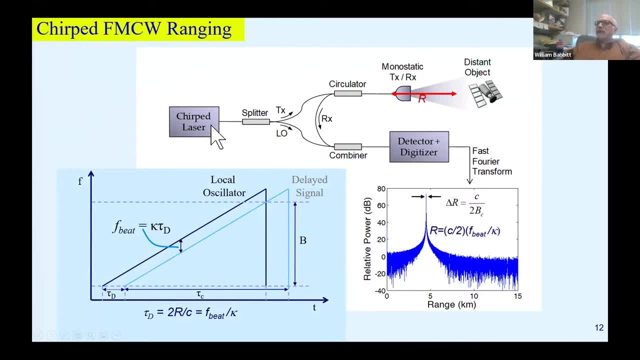 let me well, let me talk about this a little bit. let me talk about the experiment first. or the typical setup is a chirp laser. you split that into a transmit in an LO. you send the transmit out through a circulator. circulator is nice, because the the transmitted pulse goes out and the return pulse comes back. 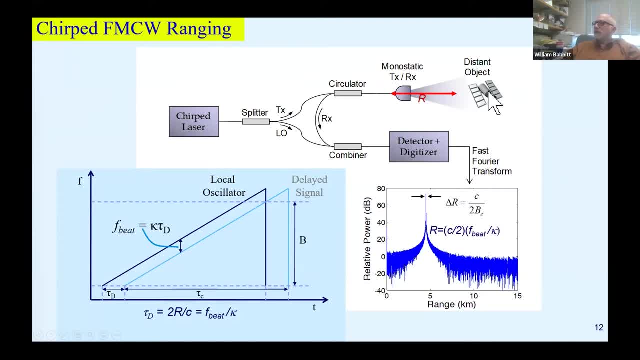 on a different path. so the pulse transmit, pulse goes out and comes back and beats with the LO and then you digitize that and I'll talk a little bit about the requirements on the digitizer and the detector- and then you for a transform it. so you send out a chirp. it comes back as a delayed chirp. 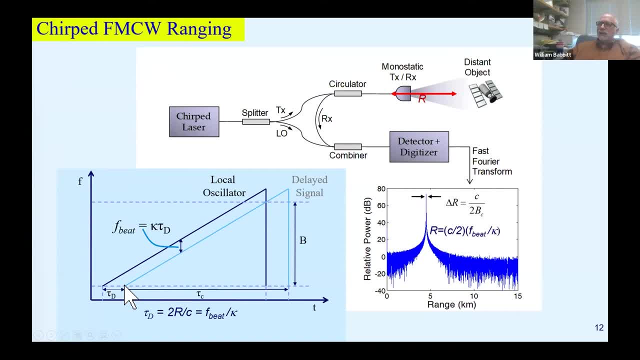 and so a delay in time here causes a frequency change between those two, between the laser and the transmitted pulse and the return pulse- this the beat frequency capital, and because that's a linear chirp, that frequency beat is constant. so you get a constant tone during the whole pulse, and if you take a for a transform, 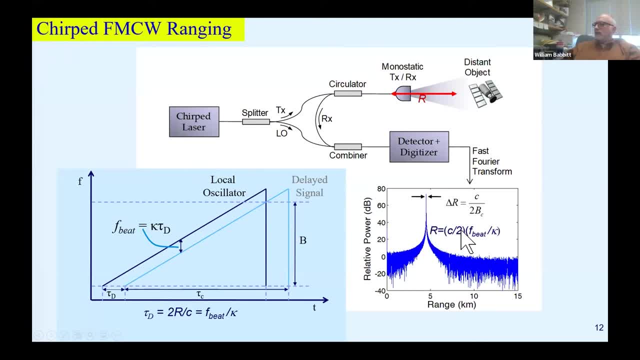 of that you'll get a beat frequency that can be multiplied and converted to a range, and so here's your fast for a transform. converted units to range and you get a very nice sharp pulse with a range resolution that is C, over two times the bandwidth, which is the same range resolution we had with pulsed LiDAR C. 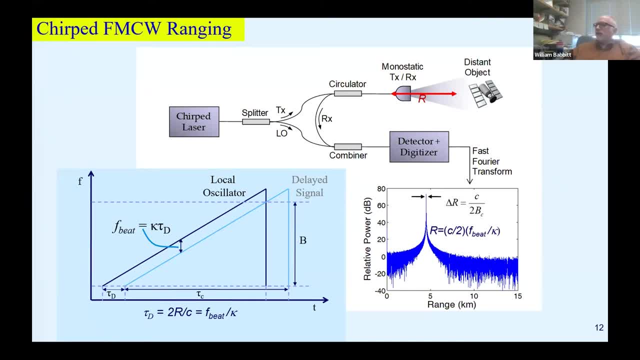 over tau, two times the bandwidth of the brief pulse, but now we have a pulse that's much longer than what it would take, much longer than a brief pulse. it all, the the range resolution, all comes from the bandwidth, not the duration, the duration of the pulse actually. 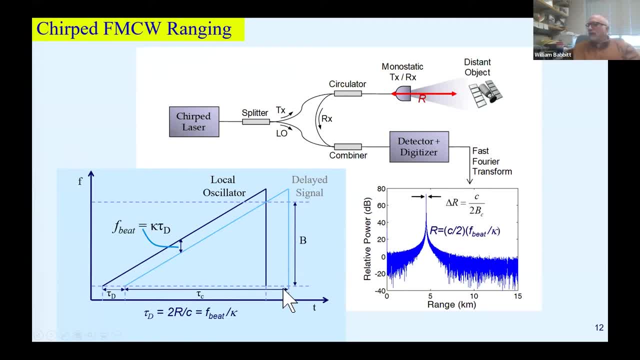 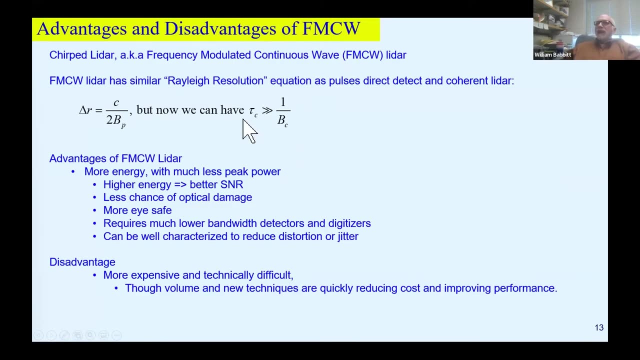 duration of the pulse. let's see here. duration of the pulse comes in in terms of kappa here and your ability to measure that frequency. well, all right, so what are the advantages and disadvantages of FMCW, LiDAR? so now we've got this range resolution. that's a function of your chirp, but now you can have. 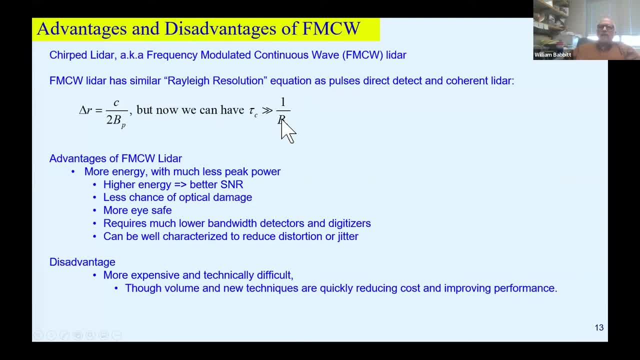 durations that are much longer than one over the bandwidth. You can have like a multi gigahertz chirp over a millisecond timescale, So you can have a factor of thousand. The duration can be on the order of a thousand, a million times one over the bandwidth. 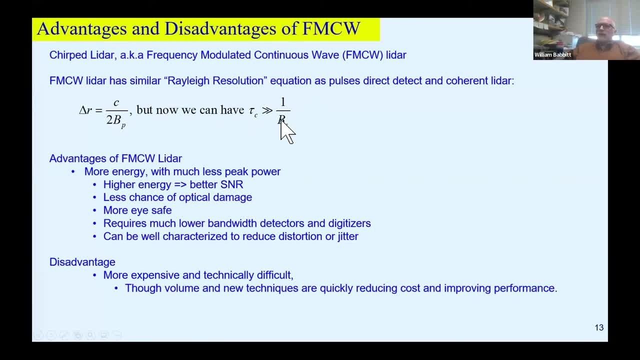 That's typical. We can do anything from a thousand to a million times. What that allows you to do is to put a lot more energy on the target without having much peak power. The peak power can be really weak. You have a long pulse. get a lot of energy on the pulse. 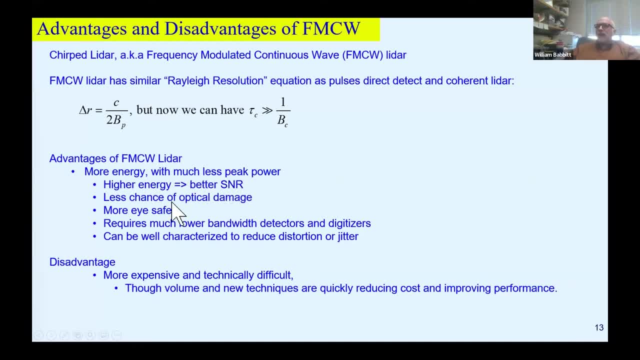 And so that higher energy gets you better SNR. There's less chance of optical damage because you're relatively weak pulses I mean you can. you can have a watt signal, but if you take a watt signal but you can have it on for a long time, 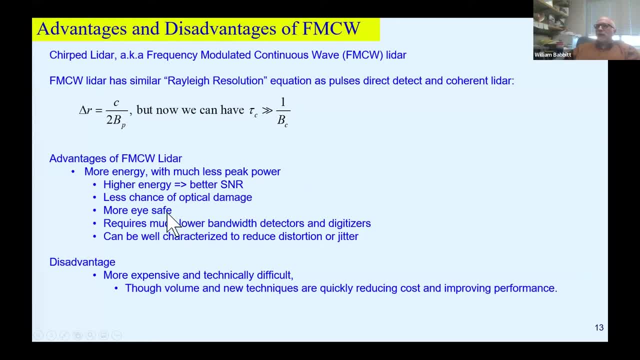 It's more safe going to long pulses rather than brief pulses. The detector requirement, the bandwidth requirement, is no longer the bandwidth of the chirp or the pulse. It's the bandwidth that allows you to get the measure, the beat frequency, So you can have much lower bandwidth. You can get high resolution with tends to. you can get the equivalent of gigahertz resolution with the order of megahertz detectors. 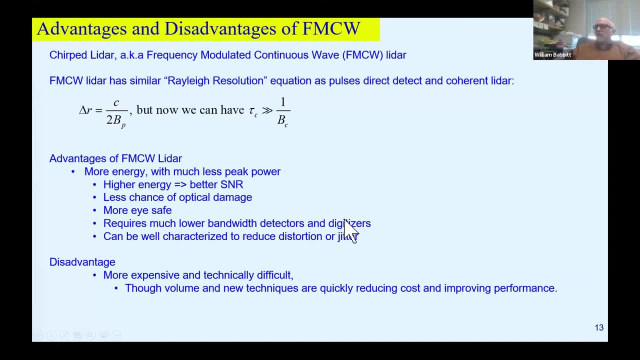 And likewise you're digitized on the same range, on the megahertz, And because they're pretty well characterized- and I'll talk about that a little bit- you have much less distortion or jitter. The disadvantage: well, they're a little bit more expensive and technically difficult to produce, but they're becoming ubiquitous. 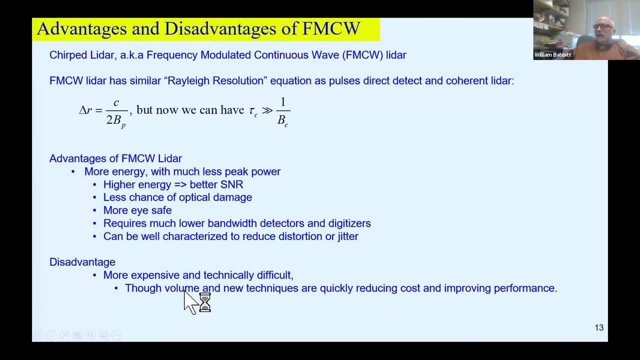 The amount of volume of FMCW sources is getting large, and there are new techniques to doing this. I'll talk about one technique, but they're more advanced techniques for producing FMCW lasers, And so the cost is coming down and the performance is getting better. 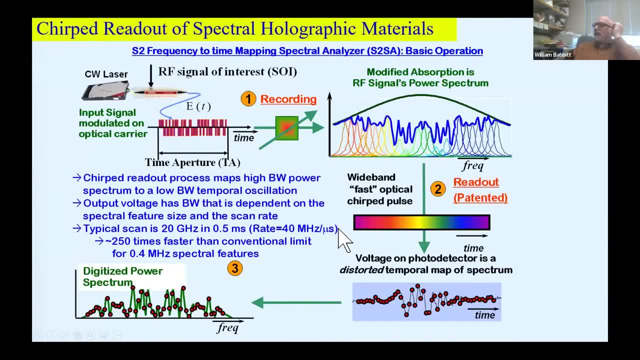 So when I first got to Montana State, I did nothing about lidar or anything like that. I was working on something called spectral holograms rather than spatial holography, And it's really a form of spectroscopy. We wanted to read out a material very quickly. 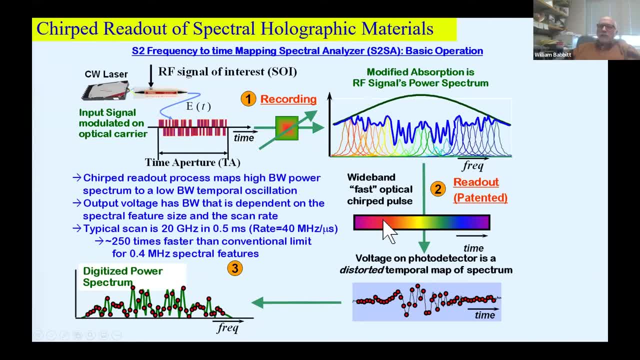 We wanted a chirp pulse that could do 10 gigahertz. We wanted a chirp pulse that could do 10 gigahertz. We wanted a chirp pulse that could do 10 gigahertz And a millisecond, And it took 10 years to develop that readout capability. 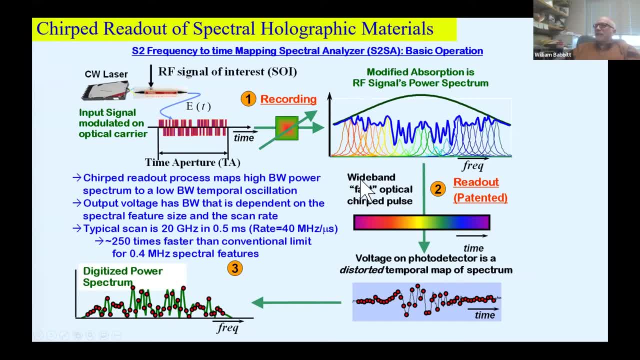 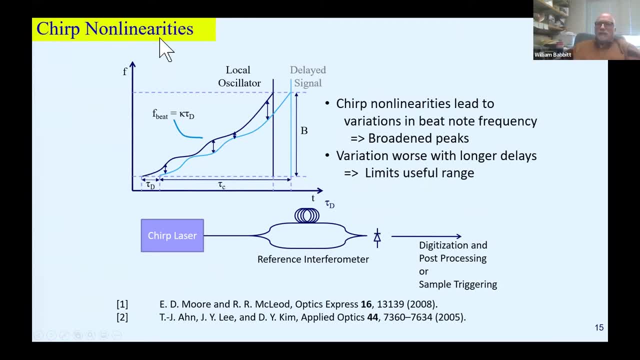 So I'm not going to go into this. I'm just saying that this is sort of the history And one of the issues we ran into is chirp nonlinearity. I mean, I was working with chirp pulses in the 80s. 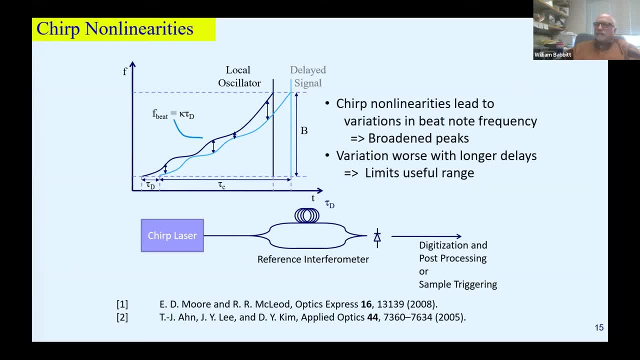 And you basically would ramp the current of your diode or change your grading. The problem is it wasn't linear And so if the chirp isn't linear, so it's doing some path and you send that out and then you get delayed return. 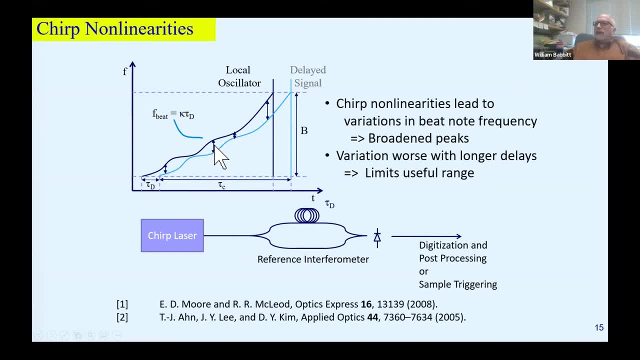 the beat frequency varies. You get a medium beat frequency, a big beat frequency, a small beat frequency, And what that does is it greatly broadens your peaks and reduces the height. So your signal is spread out and therefore your range resolution is essentially destroyed. 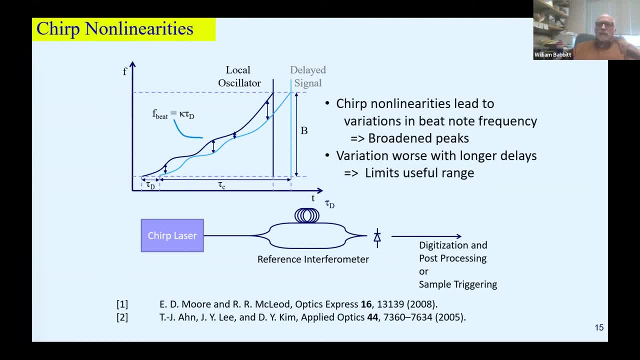 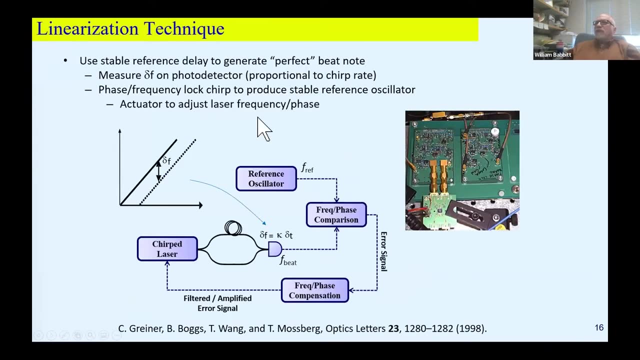 You can have a gigahertz chirp with meter type resolution, but because of the noise on it you almost have kilometer errors. It's not good, And so my- actually Tom Mossberg was my advisor when I was a graduate student. 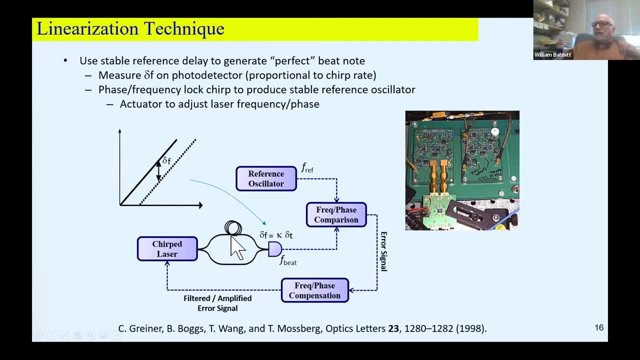 His team came up with this idea of how to stabilize the chirp. You basically you take a fibrous delay, you take your chirp and you beat it through this interferometer And you measure the beat, And as long as it doesn't actually have to be stable long, 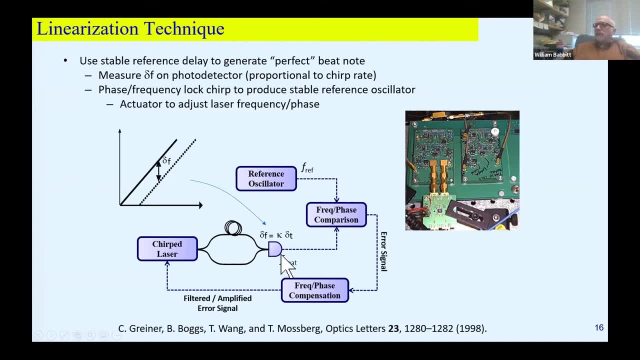 but it has to be stable during the duration of the of the chirp. You take this beat frequency and you compare it to some reference beat frequency and you feed that back so that the laser constantly keeps this beat frequency here, the same as your reference frequency. 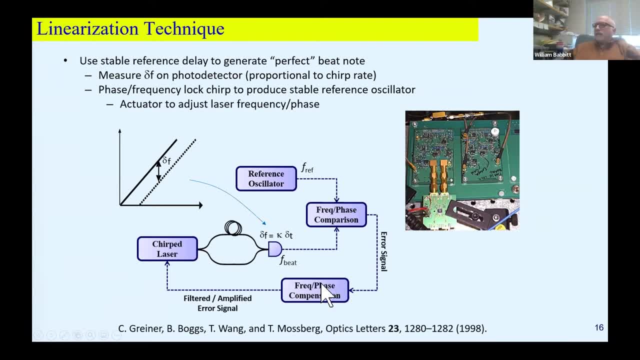 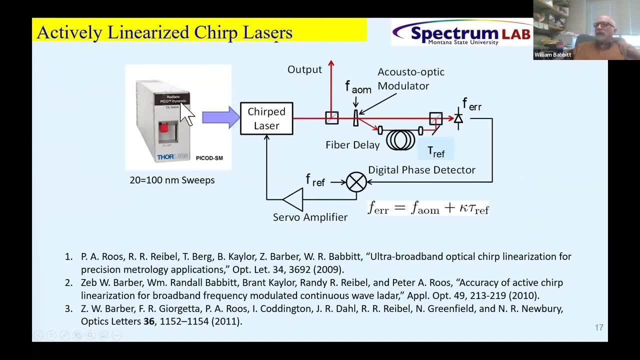 So there's a feedback system and that will linearize your chirp. We took that technique and advanced it to the point where we took a peak of D laser which can do terahertz, And so we were doing terahertz scans over milliseconds. 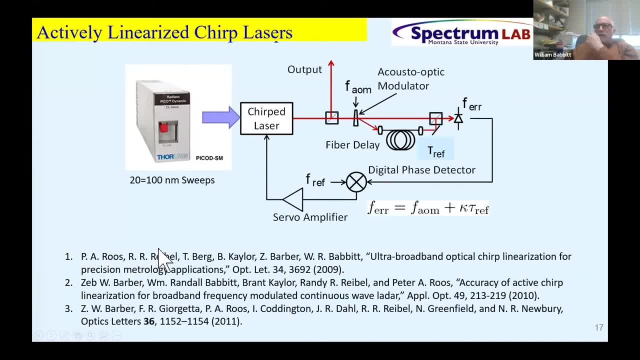 So this is actually some work done by Pete Roos and Randy Riebel. Randy was one of my students and Pete and Randy were working in Spectrum Lab. Pete's also a graduate- PhD graduate- of MSU, So was Trent was an MSU graduate. 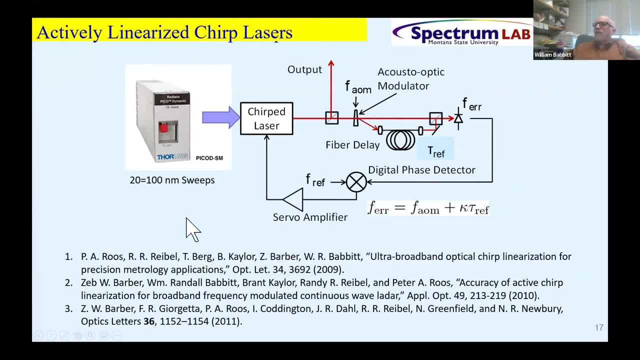 Zeb was a MSU undergraduate under CU, So all these people are MSU people graduates. They came to me and said we can not just do 10 gigahertz over a millisecond, but we can do terahertz and we can do it with sub hundred kilohertz linearization. 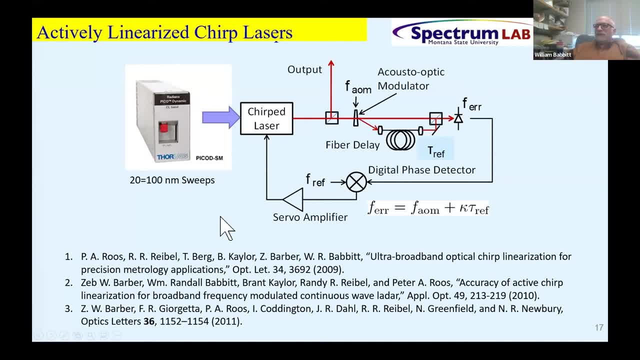 And so they came up with a technique for doing that. That was a good thing. The kind of good and bad thing was they said: well, we could care less about spectrum, Spectra, holography. We're going off and doing LIDAR work. 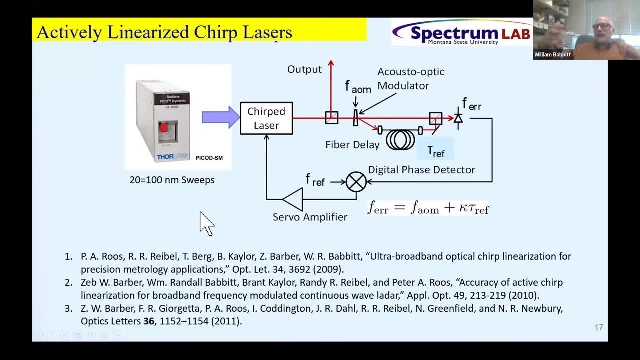 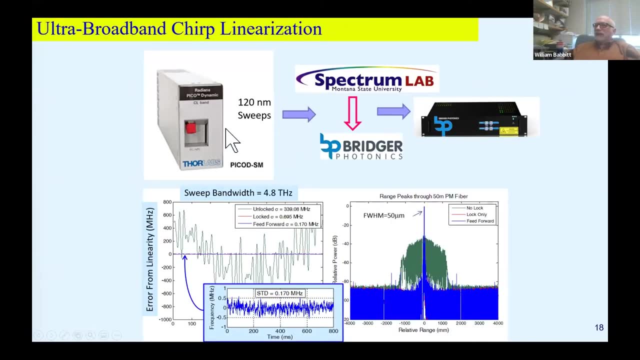 And so Randy and Pete formed Bridger Photonics, which then split off, became Blackmore Sensors, which then became Aurora. So major economic development came out of this and the Bozeman Valley, And so here's a little bit of what what that technique looked like. 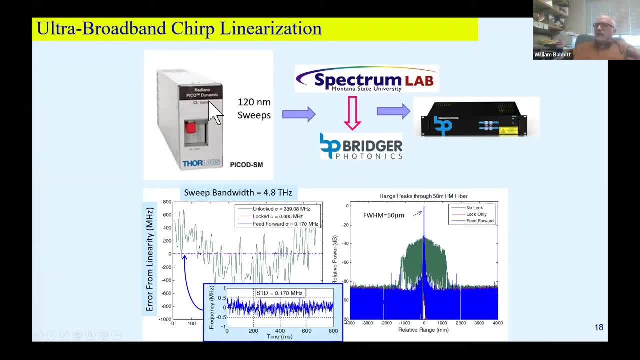 What? what the results are is that if you have a, take the peak of the laser and just sweep it, it's a grading based laser. So it's really just sweeping a grading. and you look at the linearity errors, They are on the order of half a gigahertz. 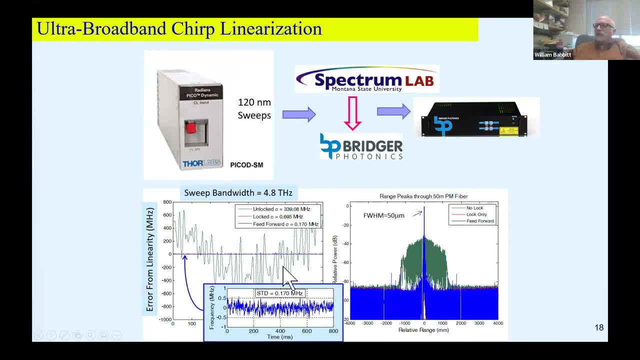 So if you just chirp the laser you'll get half gigahertz errors as you chirp in time when it's unlocked. But if you lock it, that little noise right down there- and here's a blow up of that- you can get that noise down to on the order of 100 kilohertz or better. 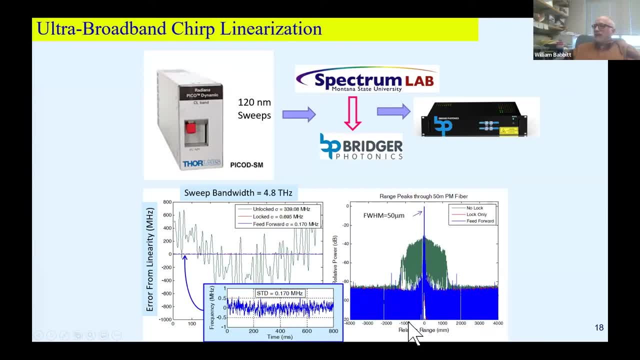 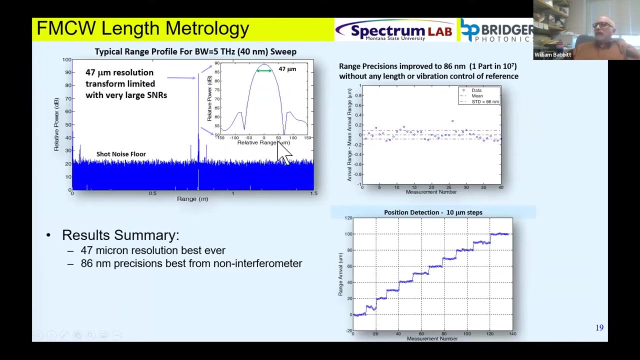 And so what that looks like in range- relative range resolution- is, rather than having when you're unlocked on the order of meter type resolutions and noisy, you get this nice spike with the order of 50 micron resolutions, equivalent 50 micron resolutions. So here's an example of that 50 micron resolution on the order. 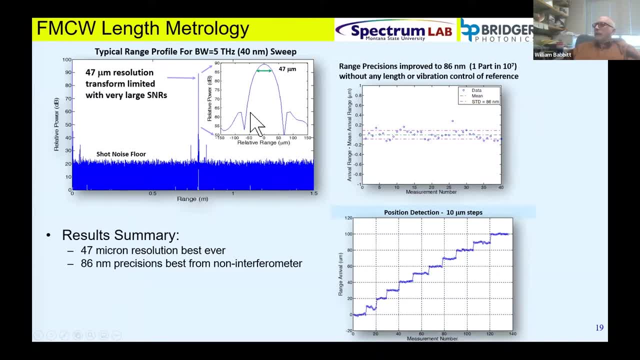 A meter timescale, a meter meter distance. They were tested that by actually moving a target with a picometer and actually show they can actually measure 10 micron steps with on the order of 47 microns resolution. They could actually do it with 86 nanometers of precision. 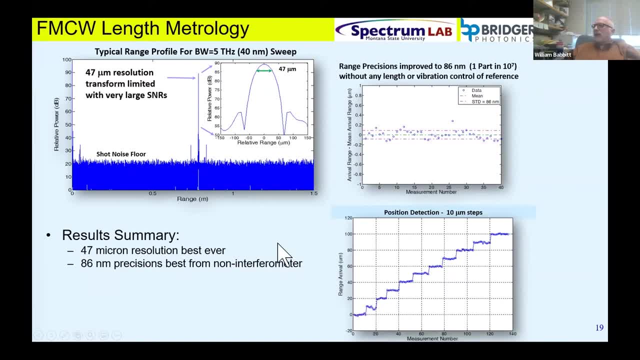 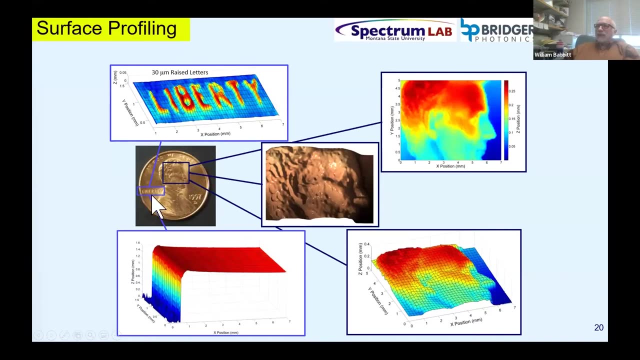 which means that because they knew it was a single target, they could come in analyze the position of the down to 80, to the sub micron resolution. They use that for doing some fun things like profiling. They could look at a penny and look at the word liberty on the penny and get profiles of that. 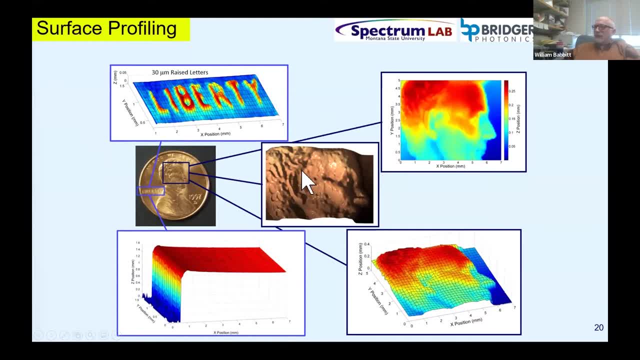 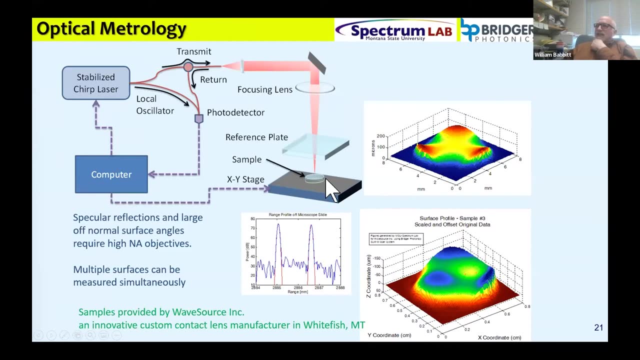 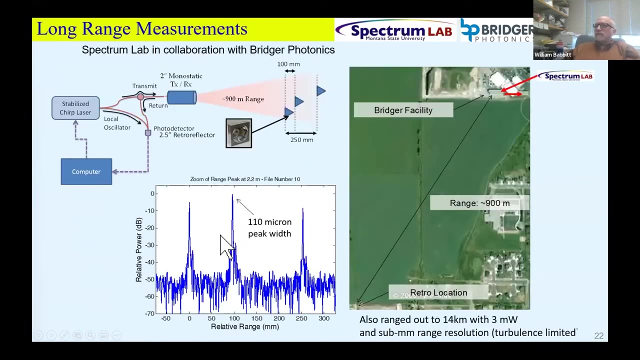 They could go into Lincoln's head and look at the wrinkles in his head and his hair. Let's see what else Let's other thing they did is they looked at contact lenses and analyze the profile of contact lenses that were being made by a Montana company called wave source. 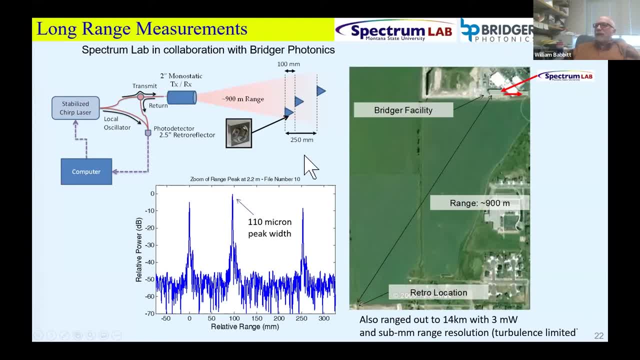 And then, oh, and they also form bridge of photonics, which we collaborated with us. They looked at long range measurements with these lidar techniques and they showed that at a kilometer they could get 100 micron peaks, 100 micron range resolutions at kilometers. 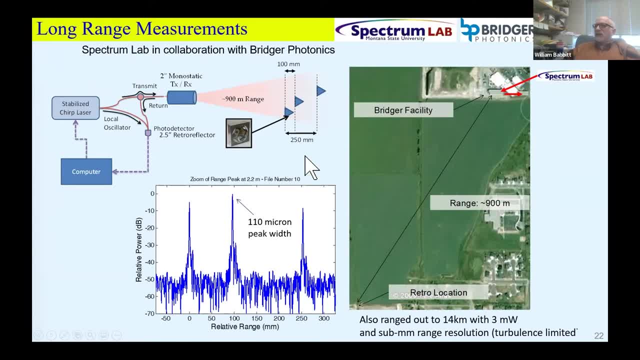 and they actually went to 14 kilometers and they could actually get some millimeter resolution And that's really was more turbulence limited And so a very precise measurements of long distance, precise and high resolution measurements at long distances. Another nice thing about FMCW: 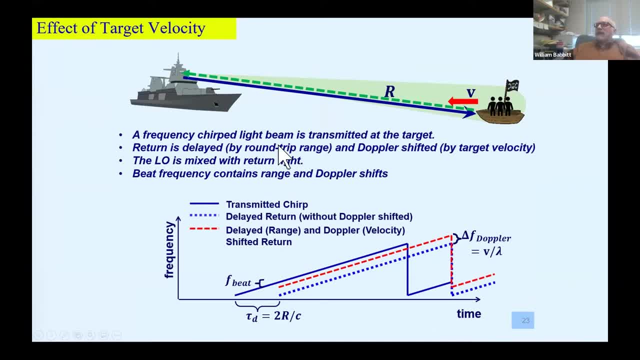 or it's good and bad thing is that the return is also the shift in the return. The beat frequency is a function of the movement of the target. And so let's say you had a target out there and it was moving towards you. that would upshift the laser. 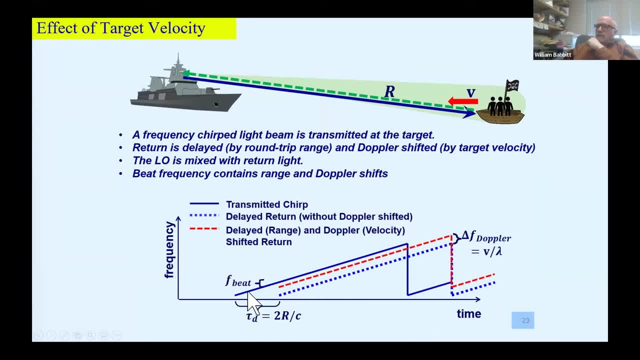 And so you get your delay causes a frequency beat. That's a function of range. But then the movement causes The Doppler shift, which also causes a shift in light. So you get a delay Shift and then a which causes a frequency beat and then a frequency shift to the Doppler. 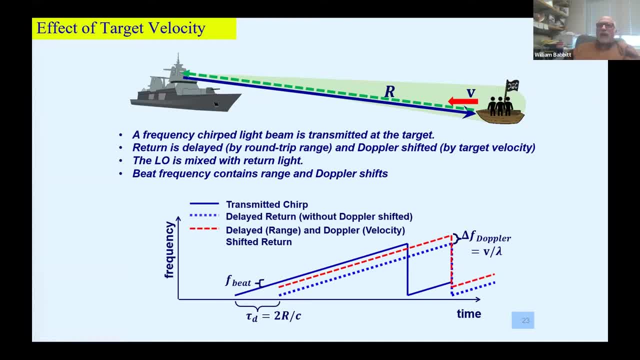 And so that can give you a range Doppler ambiguity. So you'll hear a lot with chirped FMCW techniques, whether it's radar or later. By the way, FMCW has been in radar for a long time and range Doppler ambiguity has been an issue. 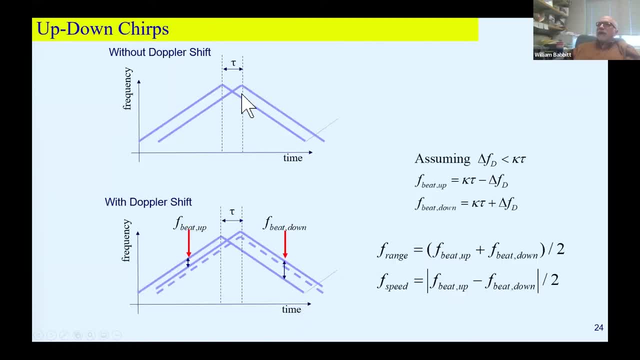 You can solve that by doing up and down chirps. And so here's a case: without the Doppler, up and down chirp, You get a. here's your transmit, Here's your return. The beat is the same when you don't have any movement. 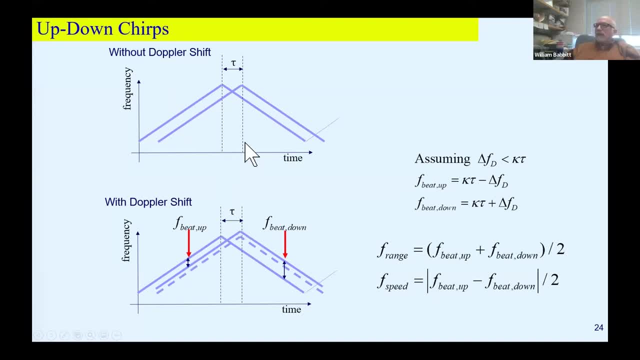 But if you have some movement of the target, then the return signal is upshifted. So here's your new return signal that's been upshifted in both locations. Well, that upshift I mean cause a reduction in the beat on the upside and an increase in the beat on the downside. 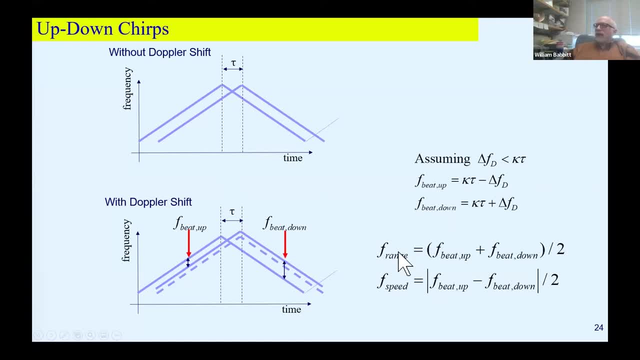 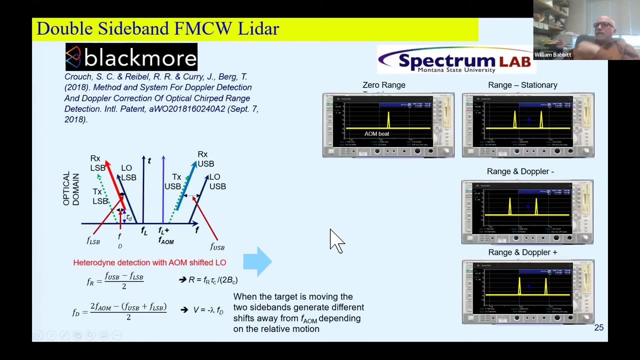 You can use that, those two measurements, to get the range beat, which is the one that's a function of capital, and the speed, which is the delta, the Doppler shift, So you can use the up and the down chirp to remove the range. Doppler ambiguity. 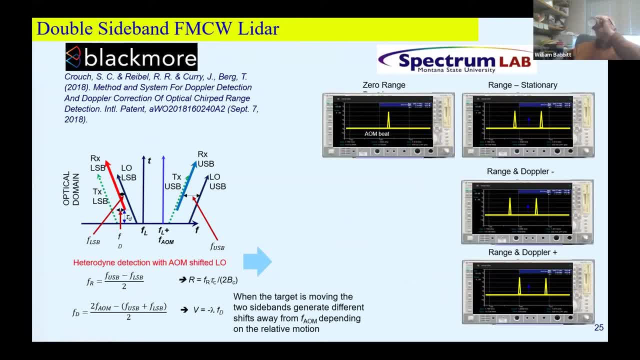 Blackmore sensors, which spun out of Bridger Photonics, became Aurora, Came up with a technique of doing double sideband FMCW. In that case you don't want to go too far in the technique, but you go into, you have a double sideband. 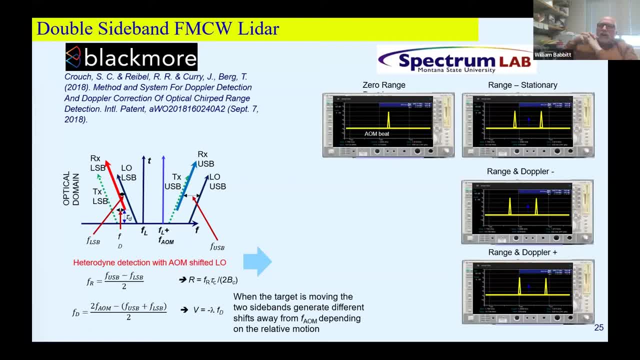 You have two sidebands, chirping which was, which would you get if you electronically chirped a electro optic modulator, phase modulator? You would get two sidebands, plus and minus sideband. You add a frequency shift- Well, that acoustic modulator- and you go through all the math. and I'm not going to go through all this. 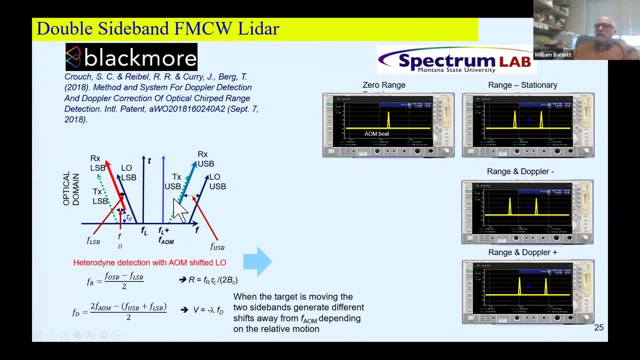 You can look at their patent, but from this one measurement, rather than having to do an up and a down. in a single measurement you get two peaks And if the target stationary, you get these two peaks. If the Doppler moves, 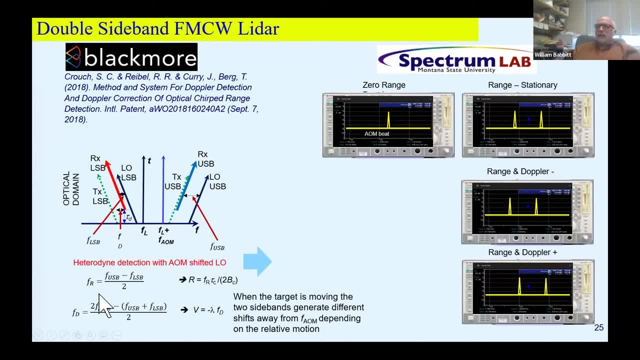 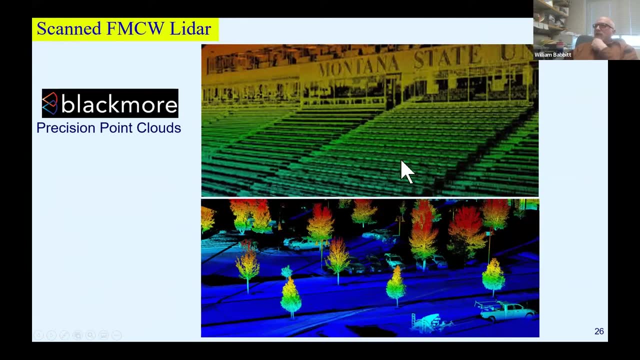 if there's Doppler shift, you see a shift one way to shift the other. You can analyze those peaks to get the same information in a single measurement. They took that technique and did a lot of interesting things. First, with just regular scanned FMCW of stationary targets. 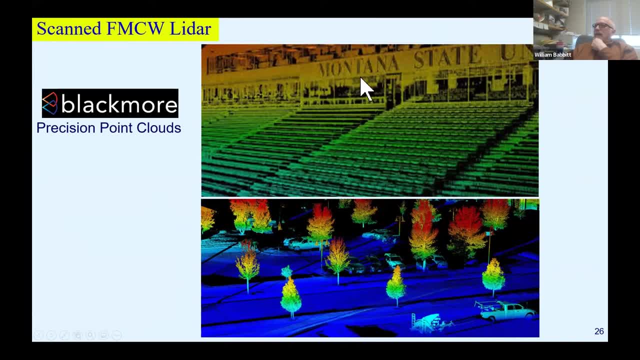 they showed the high precision they could get. Here is the Montana State Stadium. This isn't just a picture, This is a point cloud of a scanned FMCW system where they've measured the distance to every point here and plotted it. And the nice thing about these: 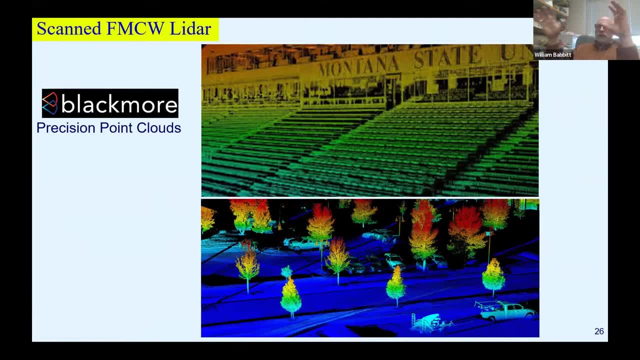 I don't have any movies of this in particular, but you can rotate this and look at it in 3D. Likewise here: you can rotate this and look at it in 3D. One reason: you can see that this is 3D. 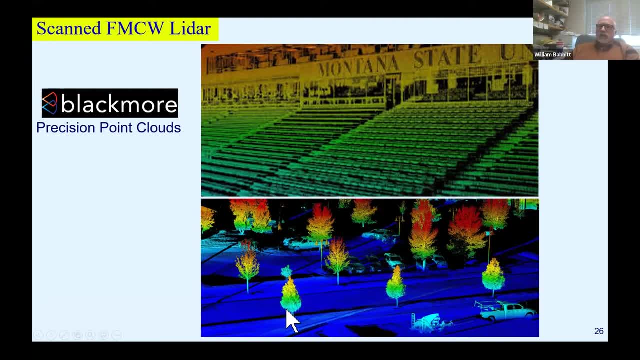 you can see the shadows. you see here not the shadows of the sun, but the shadows of the LIDAR. So this LIDAR was sitting over here and going this way. The LIDAR was really over this way, but then they were able to turn the image after the fact. 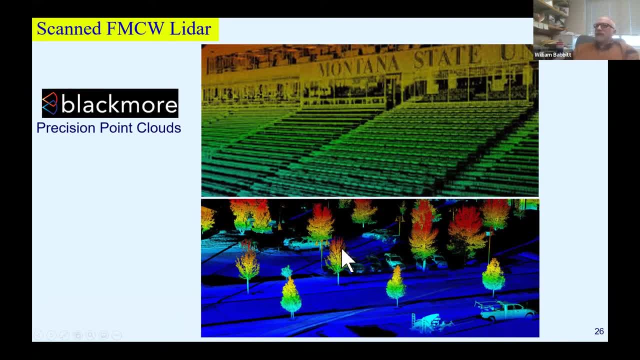 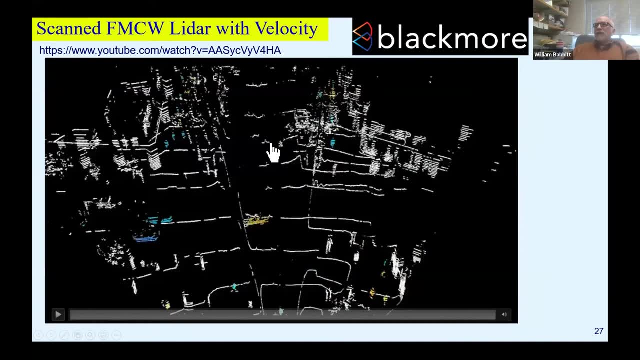 the point cloud and look at it from a different angle. So that's one nice thing about the point clouds that you can make with FMCWs. You can turn it all around. You get great 3D. Here's another thing they were doing. 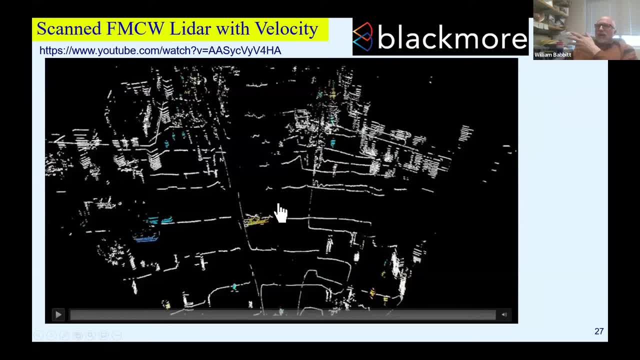 So they took this and they showed that they could do the range and velocity. And Blackmoor became Aurora, which is very much into automotive LIDAR, which Joe was talking about the other day, And this is an interesting thing where you can see the cars going by- 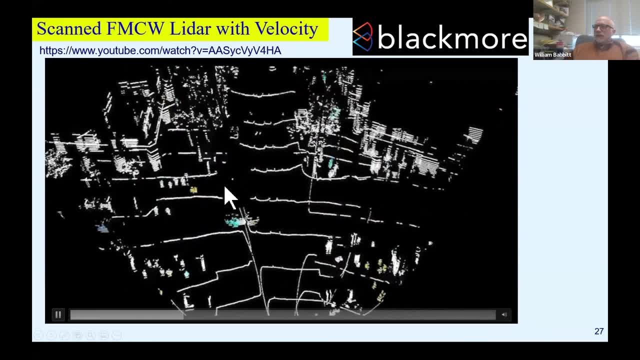 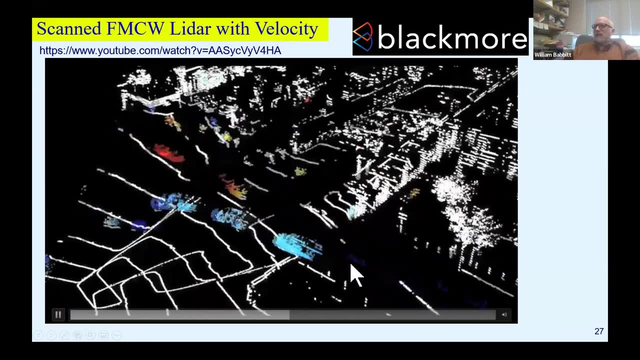 You can see people walking by And what you'll see is that sometimes the people turn blue or red. Well, that's the question of whether they're going towards you or away from you. So you can actually see the velocities. Here's the LIDAR, here. 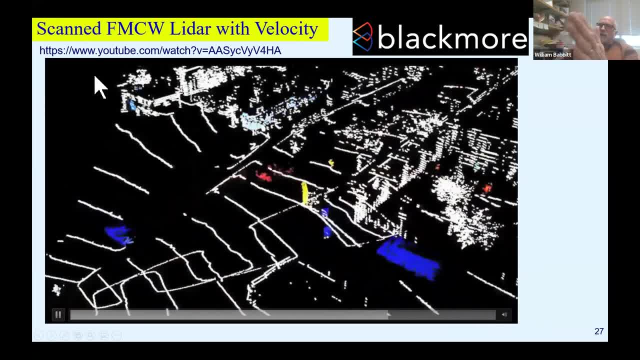 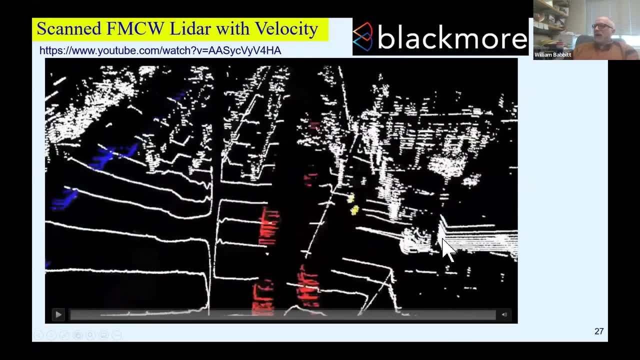 This is blue coming towards the line of sight and red as you go away from it. So it's going away as red, blue coming towards you. Things that are moving across range stay white, And so you can get the range Doppler velocity. 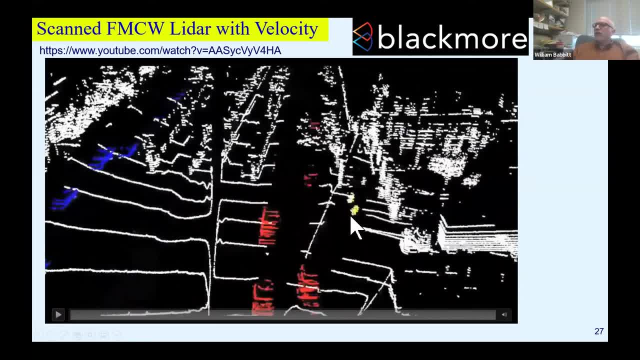 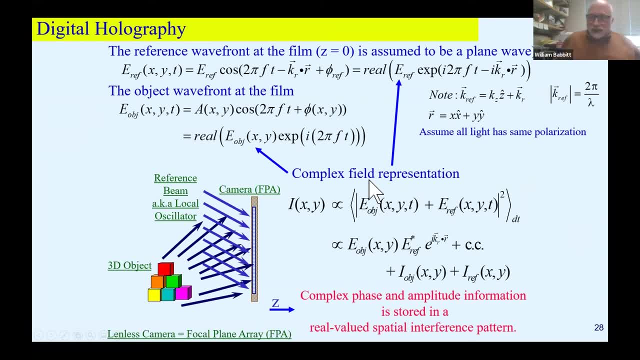 And so this is the basis of a lot of their work on automotive LIDAR. And how do I get beyond that? There we go. All right. now let's totally shift gears to digital holography. But are there any questions about the FMCW at this point? 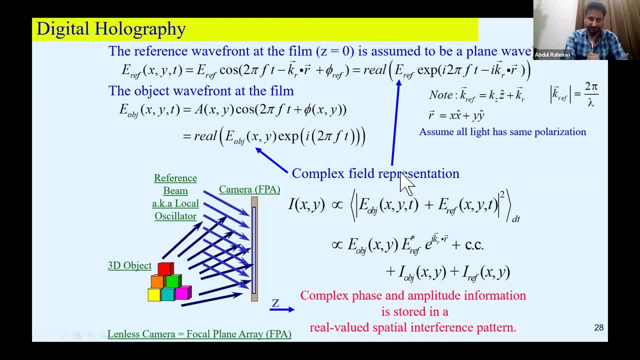 No, Randall, thank you For now. there is no question. Okay so let's totally shift gears to digital holography And let's cover all of digital holography in about 15 minutes. Okay so in digital holography. 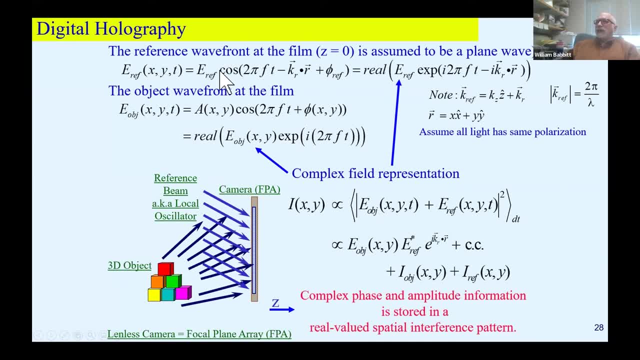 you also send out a a field to hit a target And that hits an object And the light field comes in and hits the camera, And so at the same time that a reference beam, So we have a reference beam which we can describe as an E field. 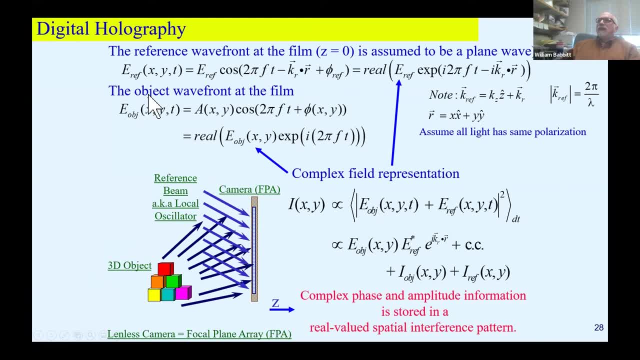 a constant E field times a cosine plane wave. The object beam is much more complicated. It's some optical field. We don't actually know its direction. It's just some complicated phase at the camera With some complicated amplitude, And this is the thing we're trying to measure. 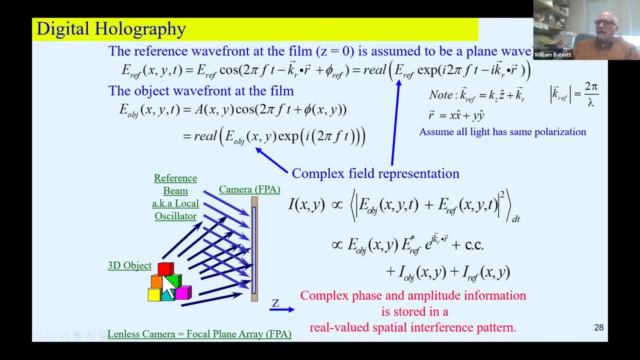 What is the amplitude XY and the phase XY of this field that is scattered from this object. And we do that by interfering that object field with the reference field. We beat those together, We capture the intensity, And again the intensity is the time averaged square of the sum of the object in the reference. 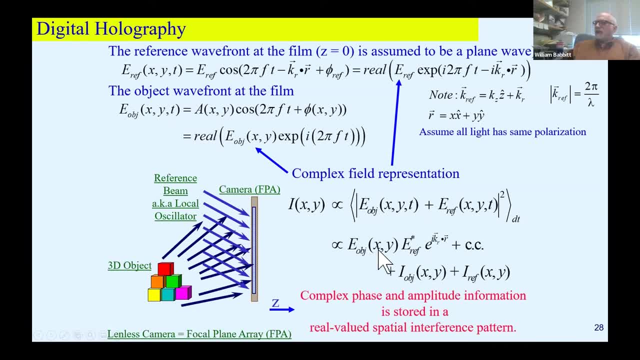 And if you look at the cross terms or the cross terms on that, you actually have a multiplication of the object field with the reference field. You have some DC terms here which we typically ignore, because we can actually filter out these DC terms Due to this modulation. 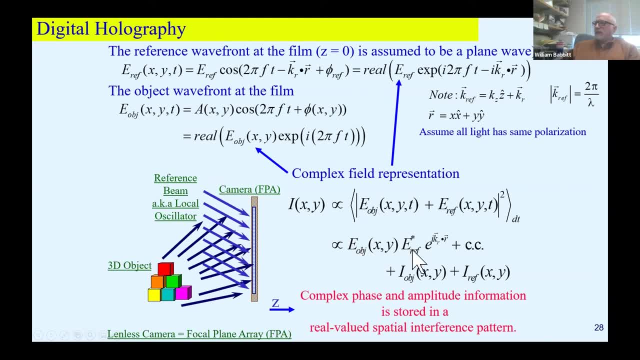 the, the electric field of the object, the electric field of reference, actually riding on a modulated background And by doing Fourier transform on that we can actually filter out the other terms, filter out this term, only pick out the terms of interest. 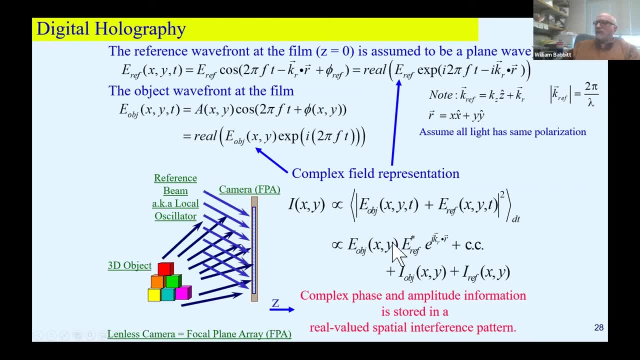 This term is actually a constant. It's the constant reference, So we can actually pick out this and I'll talk a little more about that. Oh, I just want to say whenever I say camera, I really don't mean a camera with a lens. 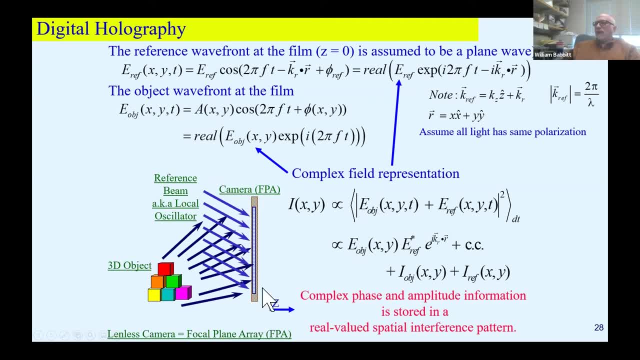 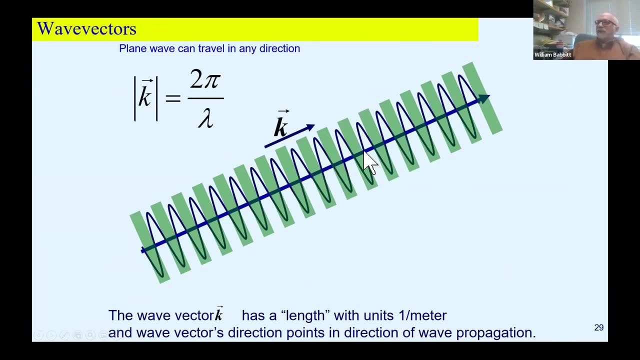 I'm talking about lensless camera or focal plane array. So when I say camera, it's really just the sensor, not the sensor plus lens. All right, So plane wave goes along. It's just a simple background. Here's a rendition of a plane wave. 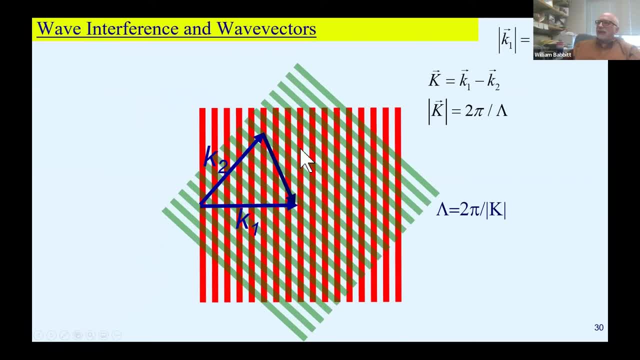 When two plane waves meet, they basically- you can see patterns here of high and low. Those are high intensity regions that form gradients with a periodicity That's actually a function of the angle at which the two meet and the wavelength of the light. 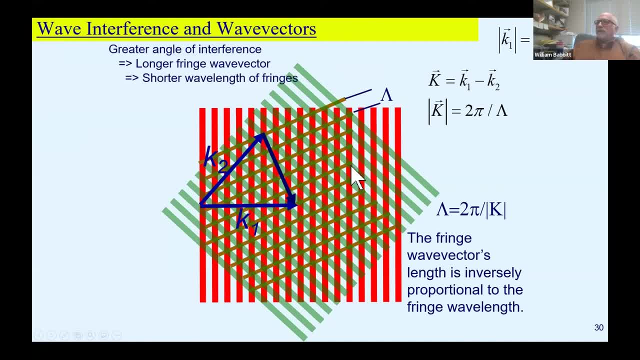 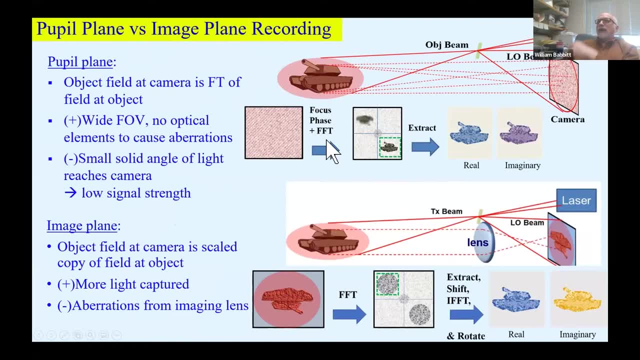 When the reference beam and the object being meet, they form thousands of gradients on the camera, And so there are two ways at which we can do the beating on the camera. We can either do it with no lens in the system, and that's called lensless holography, and also pupil plane. 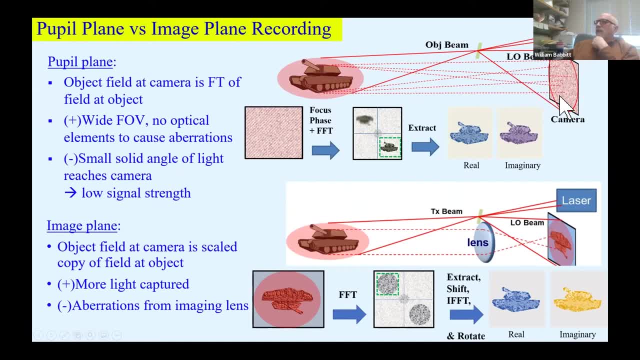 which means that really you're so far away From the target that you're really in the Fraunhofer limit here and you're looking at the people like you were in the pupil plane, or you can actually put a lens in and image the target onto the camera. 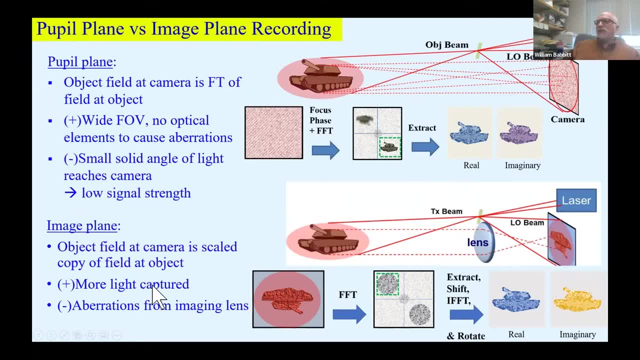 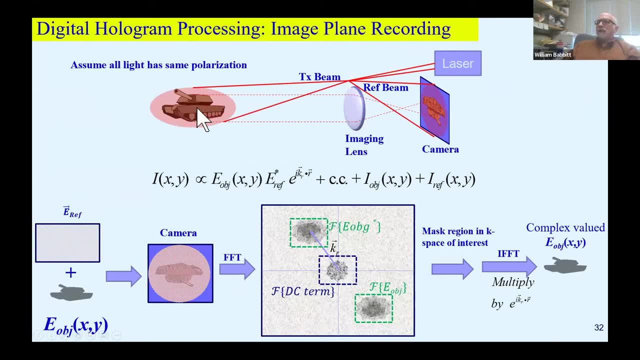 and do an image plane. I'm going to talk about image plane first and then I'll talk a little bit and talk more about pupil plane. So an image plane, you basically you're taking the target and you've imaged it onto the camera. 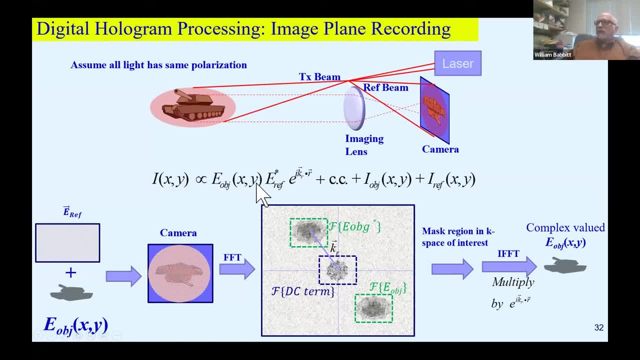 You formed a interference pattern that has an interference of the object with the reference. It's complex conjugate and then some DC terms. If you take that combination on the camera and you fast-foray transform it spatially, two-dimensional, fast-foray spatial transform. 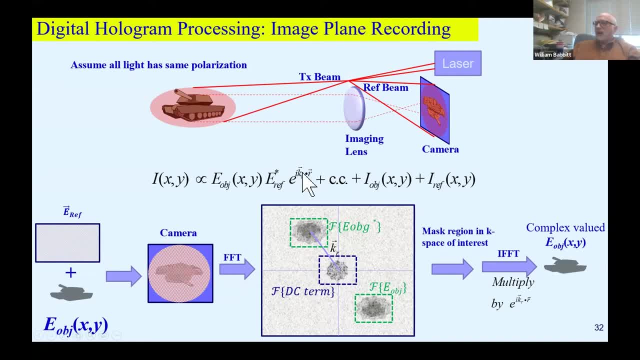 what you'll see is that, because of this k dot r term, this term shows up here, This term shows up there and the DC term show up in the center of your in the Fourier domain. If you put a mask around this blocking these two. 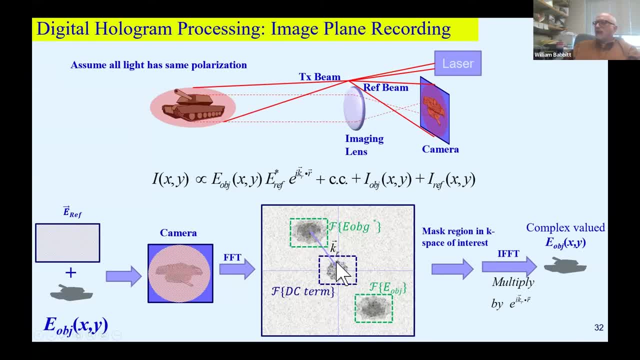 or sorry, mask around this guy. blocking these two and then inverse, Fourier, transform it, you get your target back And the nice thing is you've actually got the target, not an intensity of the target, but you have the full phase information about the complex phase information. 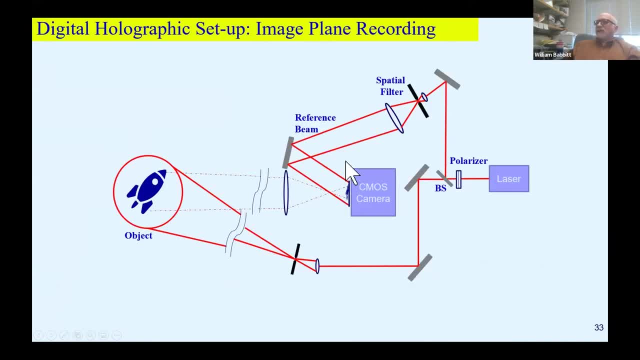 about the target. at that point Setup looks a little bit different than what I just showed you. You take a laser, You want to polarize the light because when they meet here you want them to meet with the same polarization. You form a reference beam and you want it nicely spatial, filtered on the image. 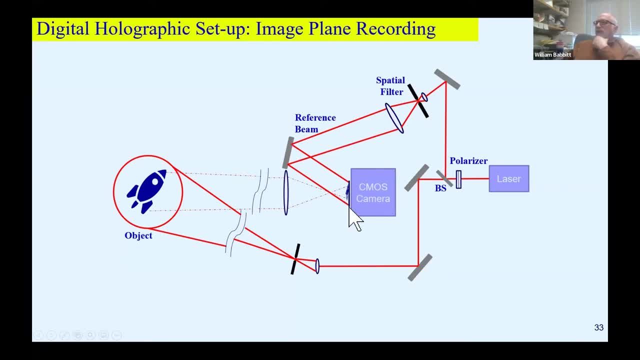 The better spatial filtering you get and the more uniform it is, the better the reconstruction. You take a transmit beam and you hit a target and then image that onto the camera And then you record that and then you do a lot of post-processing on that. 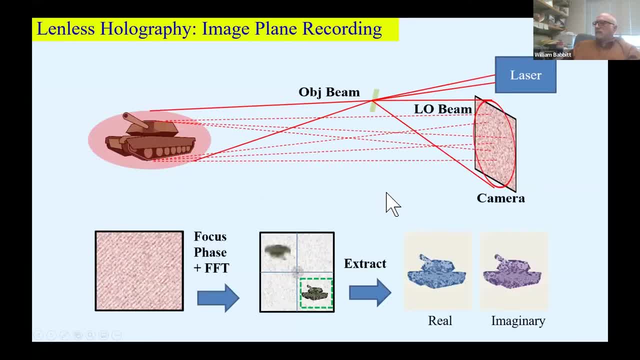 That's basically the same thing I showed a second ago. When you're doing: oh no, let's talk about that's not image plane, This is pupil plane. I'm sorry, lensless pupil plane recording. So change that word to pupil. 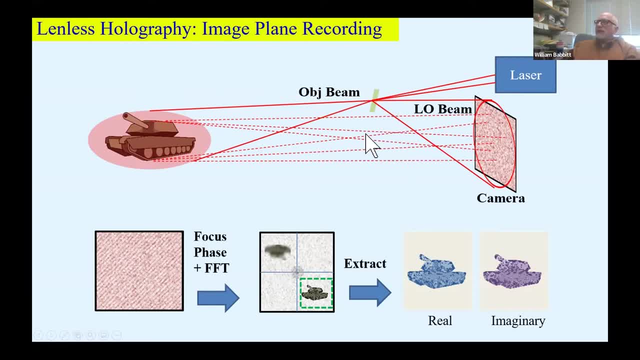 So in pupil plane we had just talked about image plane. In pupil plane there is no lens. What you see here is it's a blur of the target hitting here, beat with a reference signal. So you take that blur of the target, beat it with a reference signal. 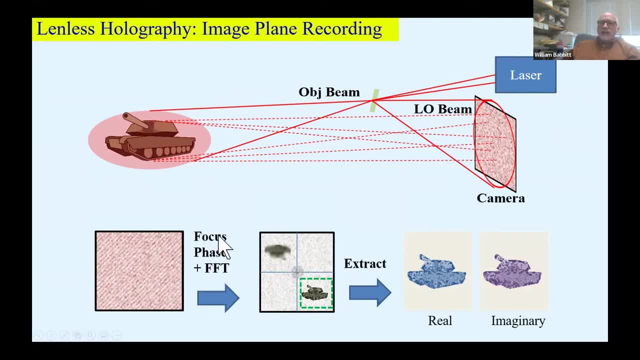 And then what you do is you add in a phase factor- which we'll talk about in a second- that focuses the beam when you do a Fourier transform and actually produces the target, And then you can mask out that and you will get the real and image part. 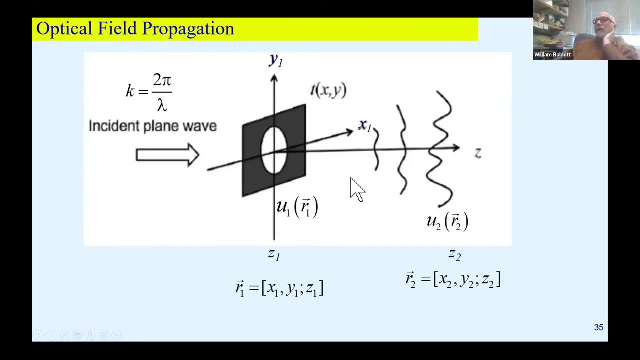 To understand this, we need to know more about how how optical field propagation works And what that. what I'm going to talk about very briefly is how to get from your object plane here- which we'll call U1, to the camera plane. 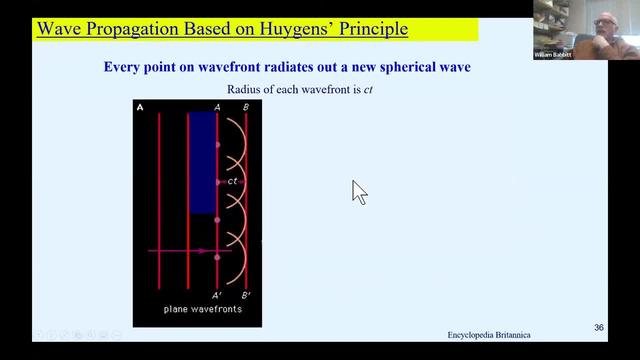 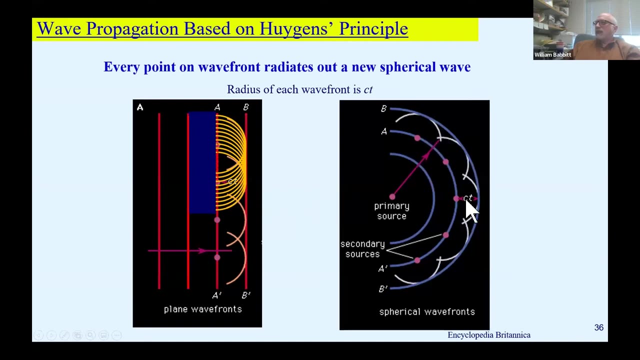 which we'll call U2. And that's based on Huygens' principle- that at every point becomes a spherical wave, And so a plane wave is really just a bunch of spherical waves that reproduce a wave front. Spherical waves work the same way. 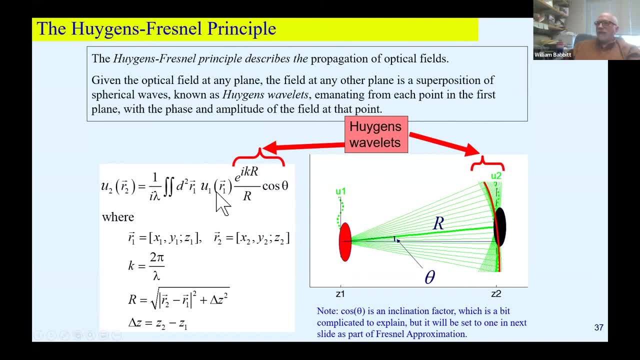 If you take Huygens' principle and you say that every point on the object becomes a spherical wave, and we tend to ignore the cosine term, which is an inclination factor which is hard to explain, but we usually just set it to one. 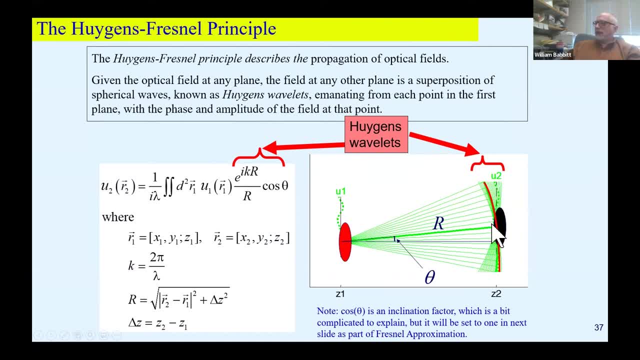 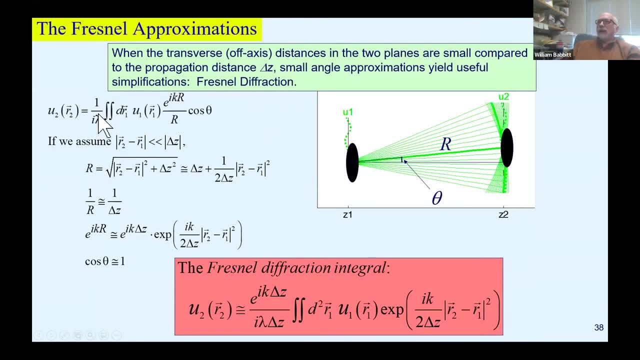 And you take this integral to get to what gets produced at the new point U2.. Then you get a, a, a. this equation here, If you make some assumptions, which is the Fresnel approximations, you assume that the range is far. 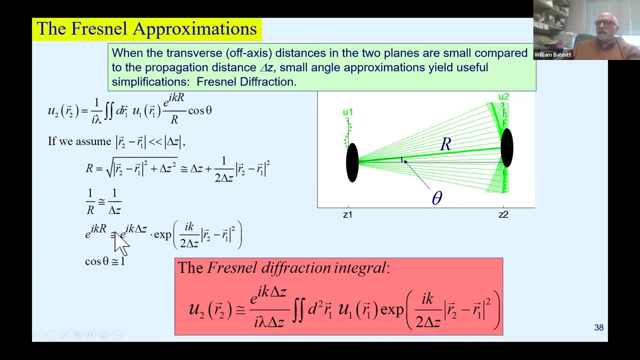 You assume that if you assume the range is far, then we can make some assumptions about K times R. We assume the cosine is one, and what we get is the Fresnel diffraction integral, And, and so you have the, the. 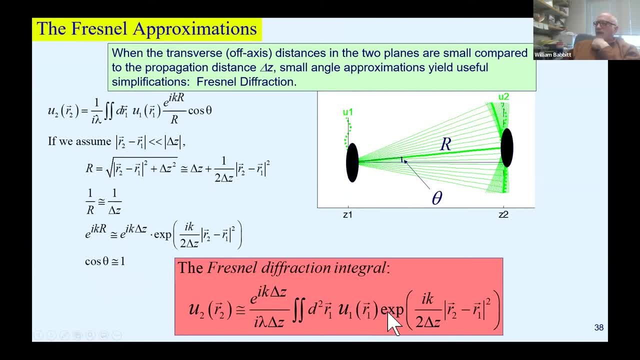 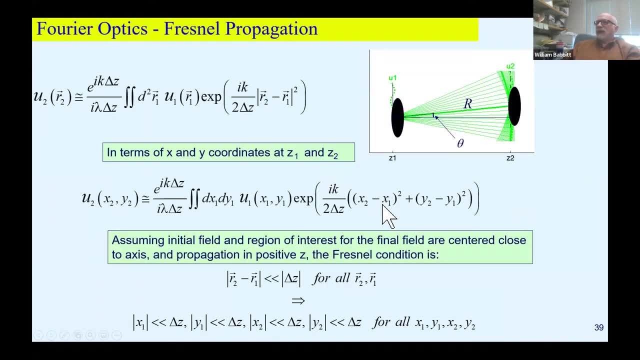 the field at U1 is multiplied times- this term here and this term here- and you get the field at U2.. You can continue to make some assumptions about that If you break this up and turn it into your XY coordinates and then you make some further assumptions. 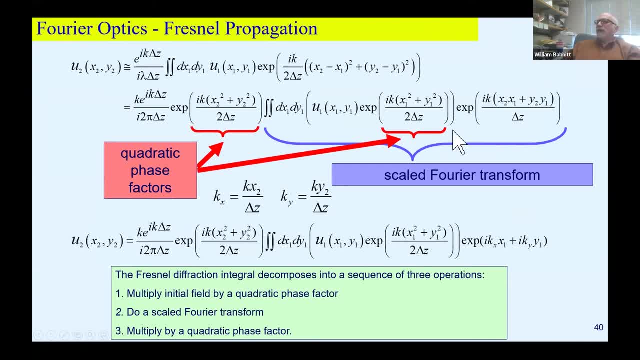 this is going to go quickly here because I'm running out of time. What you find is that in the Fresnel propagation you have the field of the object, you have a phase term, quadratic phase term multiplying the field of the object. 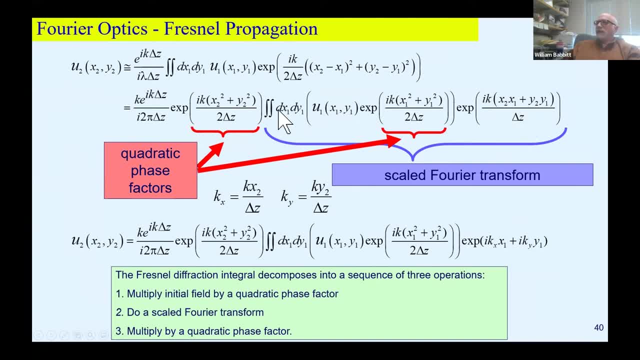 and then you have this, which looks a lot like a Fourier transform. You have the integral of dx of something that's a function of sorry dx1 and y1, something that's a function of x1 and y1, times an e to the ik. 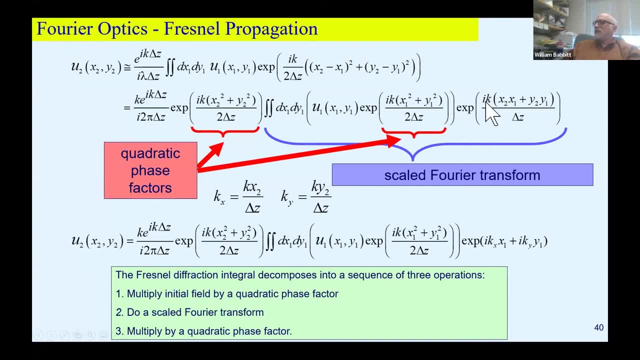 and you can think of this thing as the, the spatial frequency ik x2 over delta z is sort of a spatial frequency. So you're really doing a fast Fourier, a Fourier transform here, And then there's some quatic phase terms on the back end. 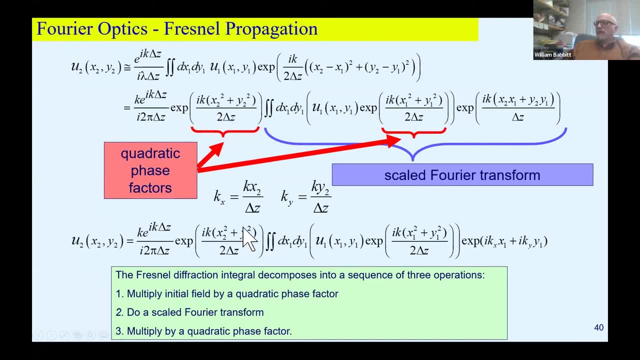 that you have to take care of as well, And so the result is really a Fourier transform of the field, with some phase terms added in. And what makes that interesting? for when you're doing? that's where it transforms when you're doing. 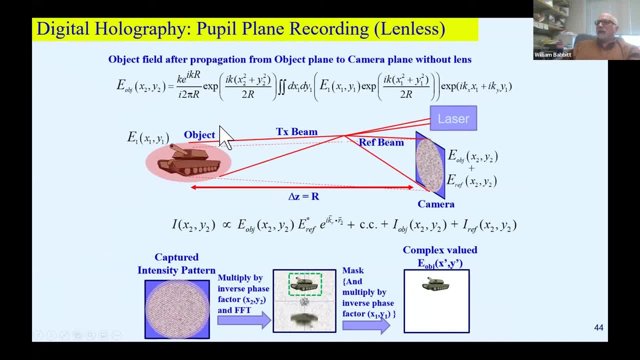 I'm not gonna do. Fraunhofer, when you're doing pupil plane and you get this return signal and you capture it with pupil plane holography, you basically can get the electric field. You can undo that. So here's the field that you would get. 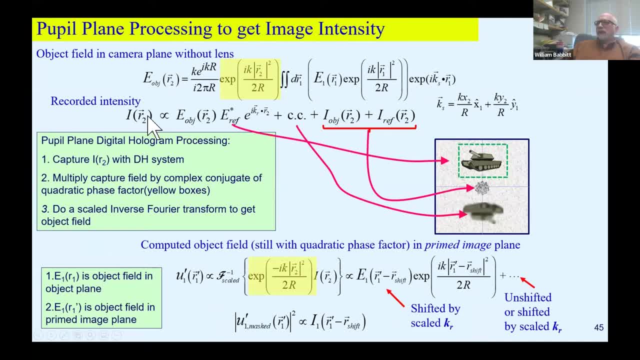 for Fresnel propagation. You record that in the intensity of your hologram and you basically pull out the e object. and you basically pull out the e object by doing the Fourier transform. But before you do that, what you do is you multiply the intensity. 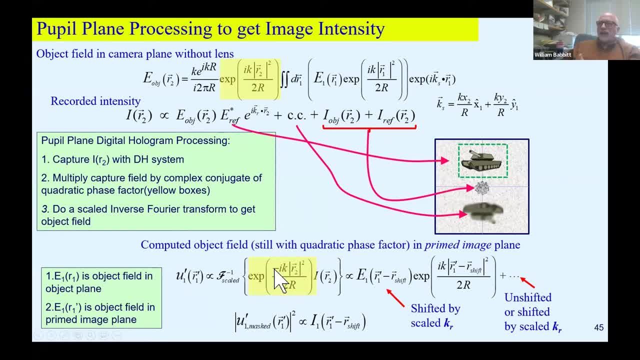 by this opposite of the scale factor, which is really a focusing factor. You undo the focusing effect and you can pull out the image. Now the interesting thing is is that that range was arranged with a target And what you do is you can pick out that. 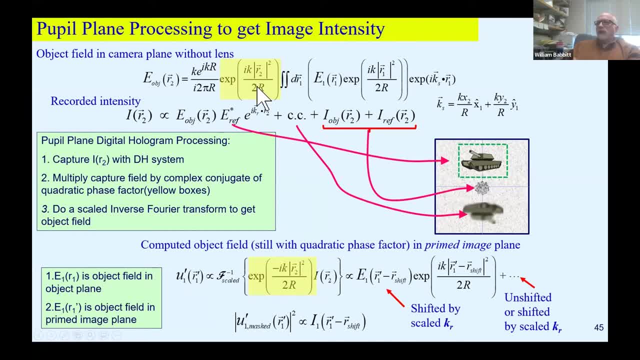 this thing picks out that range, And so you can. if there were two targets at different ranges, you can set your range here to whichever target range you want and focus that image. So you can actually focus different objects this way, but depending on what you put up front here. 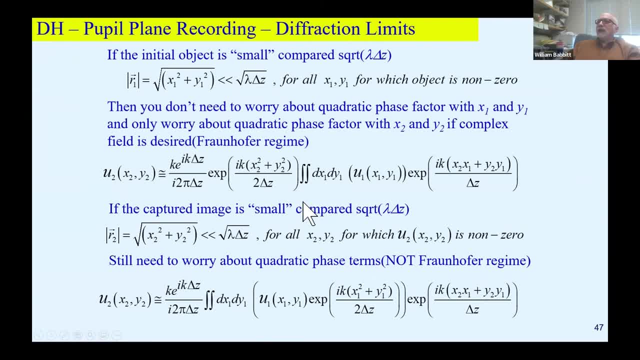 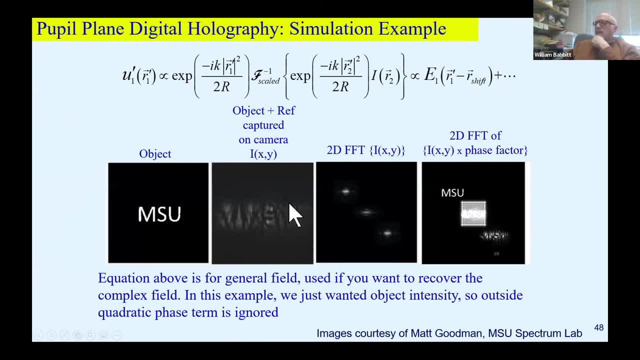 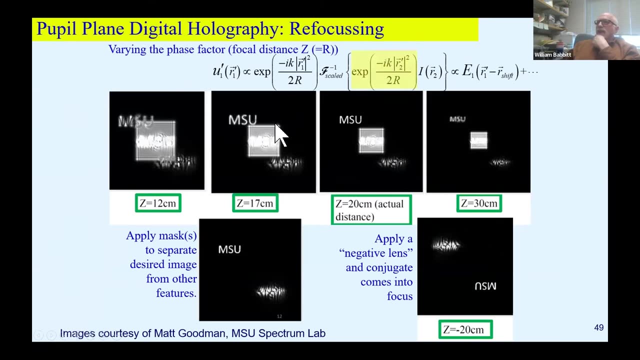 when you do the Fourier transform, Let's see, I'm not gonna go there, And so this shows you how. let's see this over here. This one shows you how you can change this focus factor. here You can actually bring targets into focus: 20 centimeters. 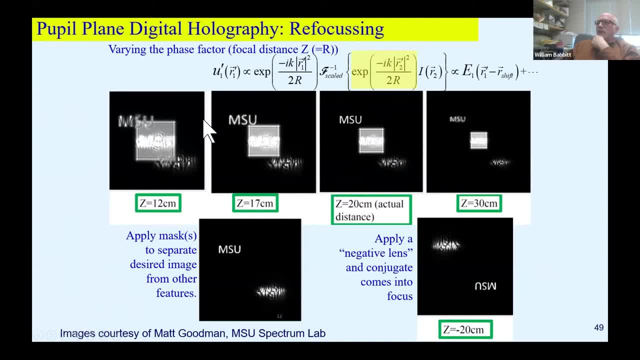 or out of focus. from 12 centimeters gets pretty blurry. up to 30 centimeters is blurry. You can change the focus of what you're focusing. If there was a target at 30 centimeters, somewhere else it would have showed up in focus. 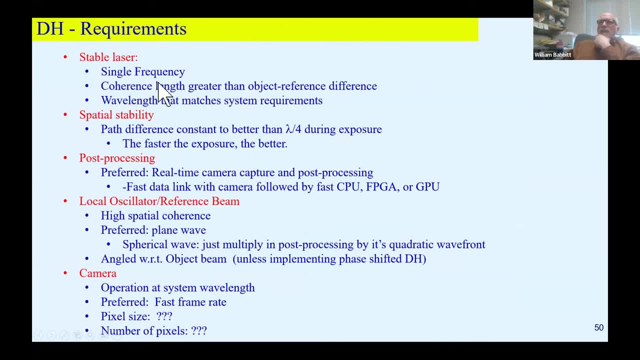 All right. digital holography requirements a stable laser Spatial stability. if your target's moving, that'll wipe out your gratings. You need some post-processing If you wanna do it real time. you better have fast CPU or FPGA or GPU on the back end. 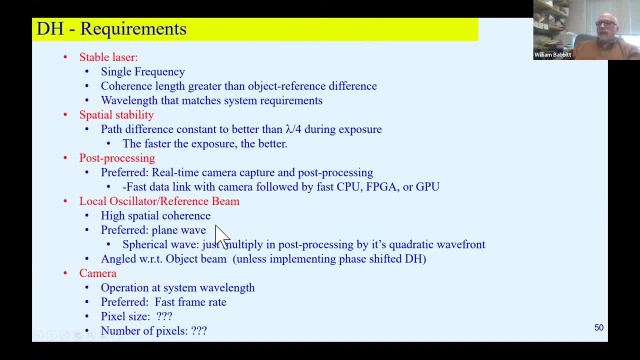 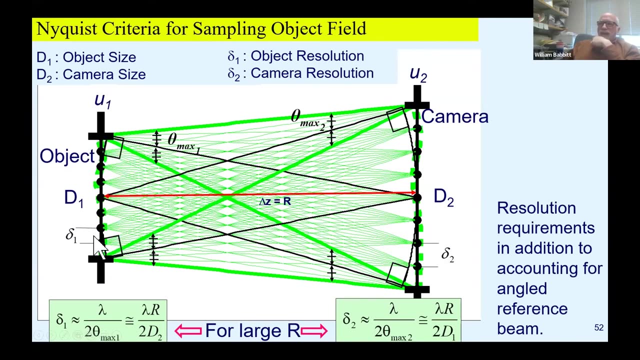 You need a good local oscillator And the camera requirements are something I'm gonna talk about very briefly. The pixel size and the number of pixels talk about that here. If you look at your object and you think about the fact that it has a resolution of your object. 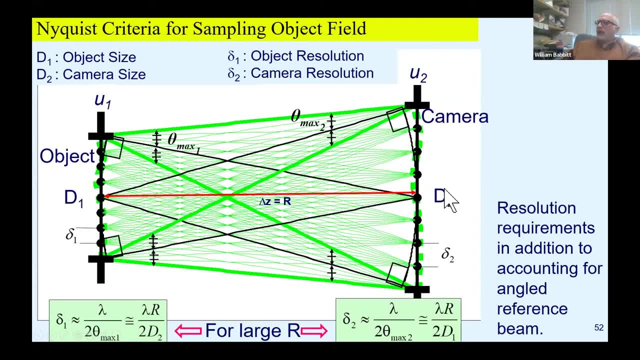 delta one and a size D1, and your camera has a size D2 and a resolution delta two, then the two things are related. The resolution here dictates the size of the camera you need. The resolution here is a function that you need over here. 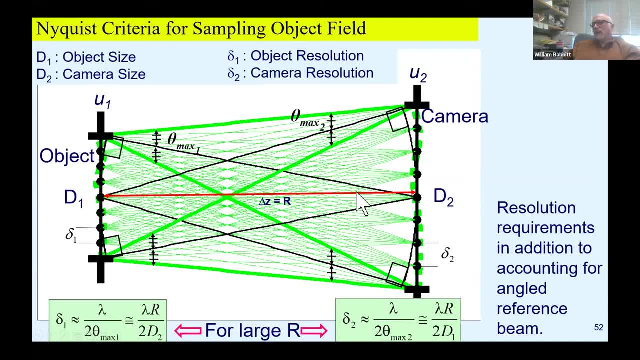 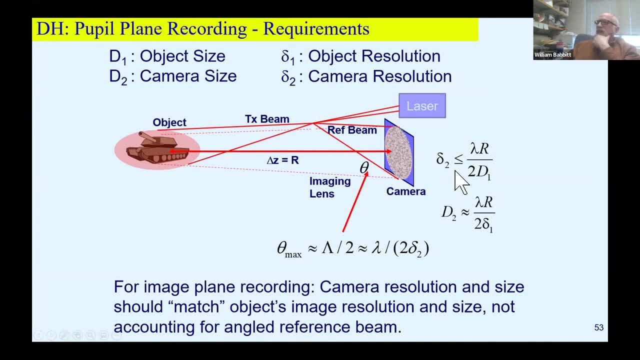 is a function of your range as well as the size over here, And so if you analyze all this, you come down to these requirements that you want the if you have an object that is size D1, at a range R and using a wavelength lambda. 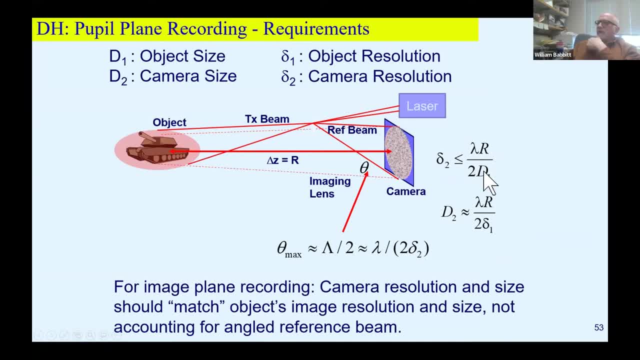 then your pixel size better be lambda R over D1.. The total camera size is a function of how big is the resolution of the target that you want to achieve. If your target had resolution delta, one that you're trying to achieve on the target, 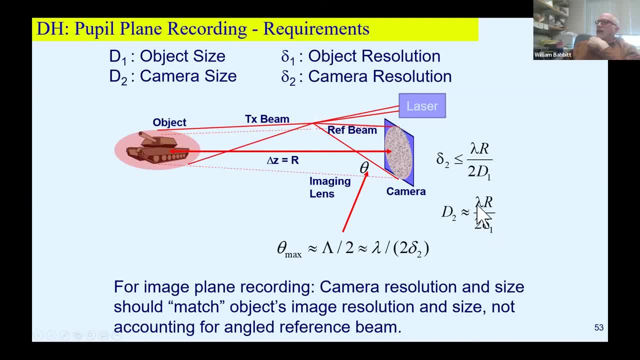 then you need a camera that is lambda R over delta one. So the higher resolution requires a bigger camera. Bigger objects require finer resolution of your pixels. That's an addition to a requirement on the angle of your object beam to your object beam to your transmit beam. 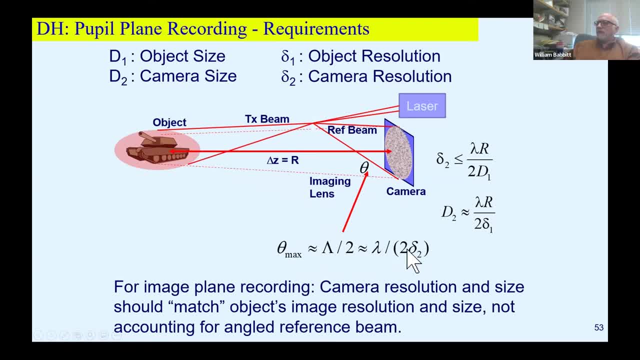 which can be a maximum of lambda over two times your pixel resolution. So your pixel resolution. remember that if the bigger the angle between your transmit and your reference and your object raises a higher resolution rating, you better have a higher resolution pixels to grab that. 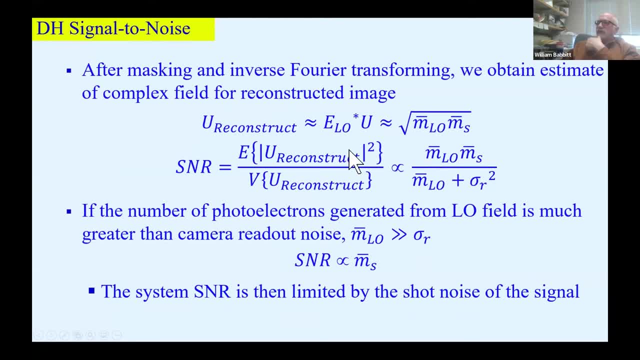 This just says that essentially the signal to noise when you're doing digital holography, if you have a strong LO, then the signal to noise, the noise on the LO, the number on the LO, cancel and you basically can get shot noise. 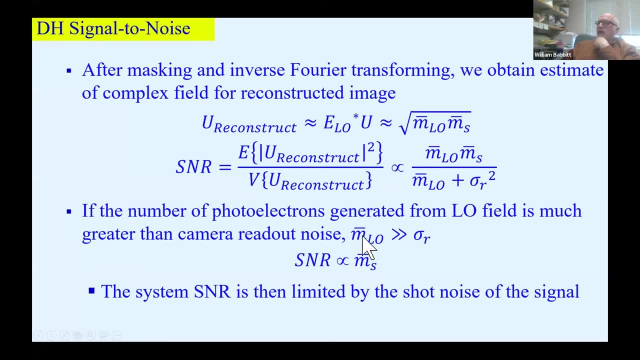 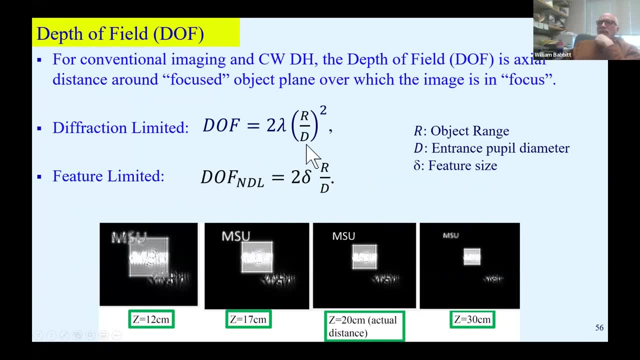 limited detection in digital holography, just like you can do in coherent detection with FMCW. Depth of field: So the depth of field of holography is really of CW holography really the same as conventional imaging, where the depth of field 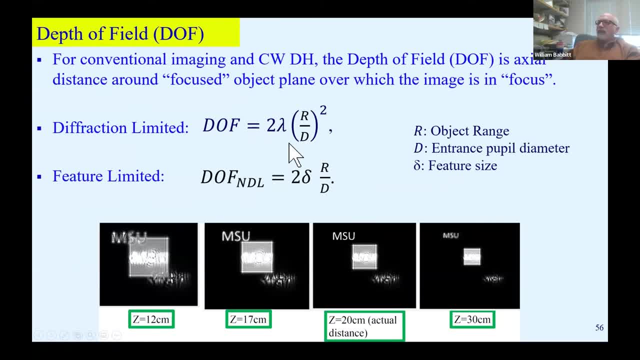 if you want to do diffraction limited is a function of the range. The longer the range, the bigger the depth of field. And what is the depth of field? It's the range over which an object appears in focus. So here's an object in focus. 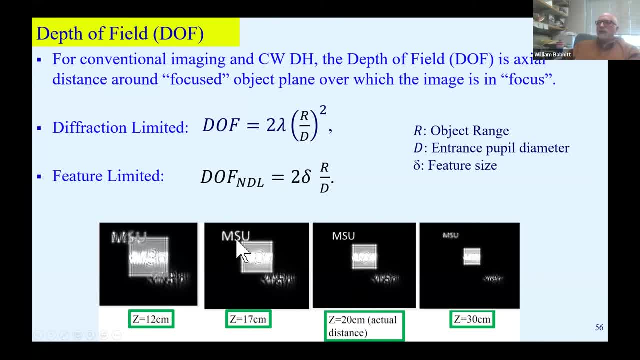 You change the range by three centimeters and it's pretty much still in focus. You continue to change it. it gets more blurred. At this point it's no longer diffraction limited depth of field, But because the feature sizes are much greater than diffraction limit. 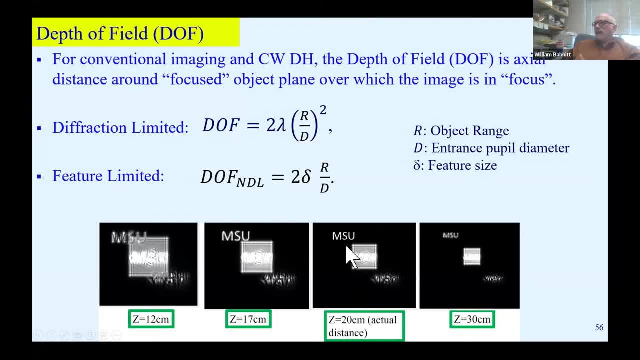 there's a thing called a feature- limited depth of field- And the one thing to go from this is if you, even though you can change your focus with digital holography, you really can't eliminate targets. They become blurs, And so if you had two targets, 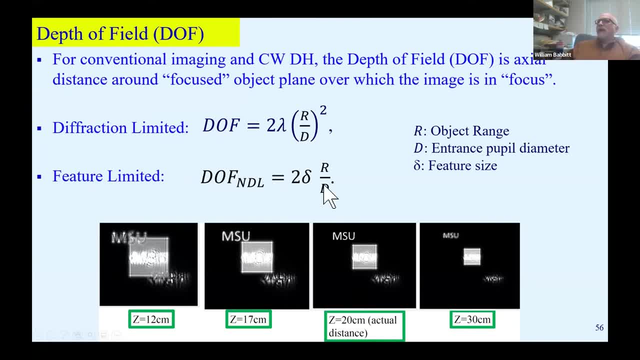 they are different ranges. it's hard to distinguish between the two, And that's why we combined FMCW with digital holography, Because we want to get not the depth of field that's of conventional holography, we want the depth of field of FMCW, LiDAR. 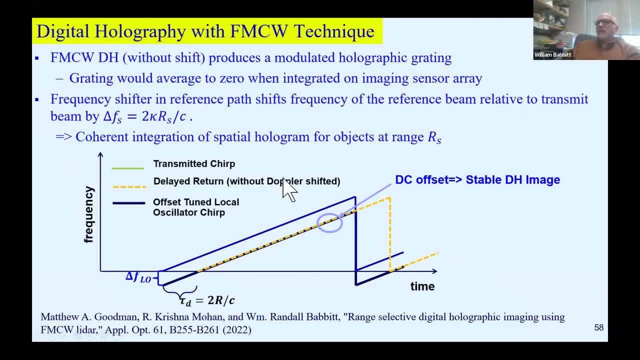 We want to get this high resolution of FMCW LiDAR. So some of the stuff we've done recently is to combine digital holography with FMCW techniques, which means that what we did is we took an FMCW beam. 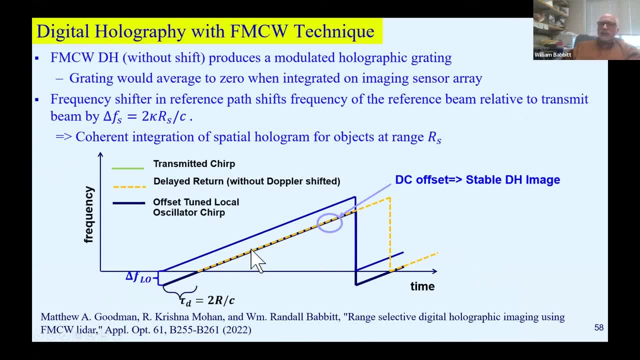 we sent it out to our target. it came back delayed. If we just put this on the camera, there would be a beat, The grating would be beating and the camera would integrate that to zero. So what we do is we then take our transmit beam and we offset it. 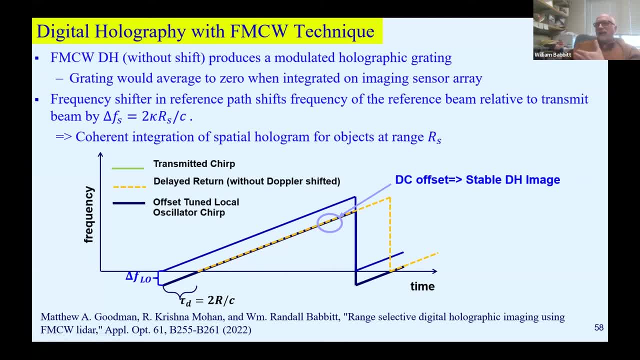 so that the beat between the return light and the LO on the camera is zero, And so we get a nice, stable hologram. Now to do that, that offset is a function of the range of the target, And so we can pick a range at which we want to look at a target. 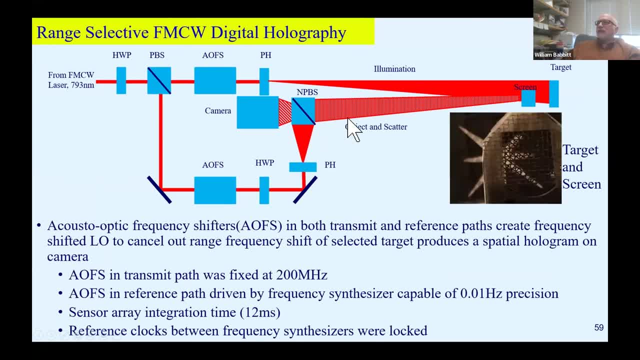 And so here is the setup that we tested this with: We have an FM, So our source is no longer a CW laser, It's a frequency modulated chirp. We send that out through two acoustic modulators, which allows us to adjust the frequency shift between the transmit and reference beam on the camera. 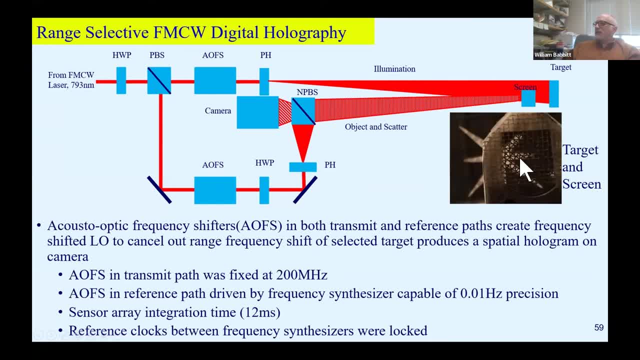 We put out two targets. One was a star pattern and 12 centimeters in front of that. We put this screen On a lens mount in front of that, And I won't go into the details, but one. if we just had the target out there. 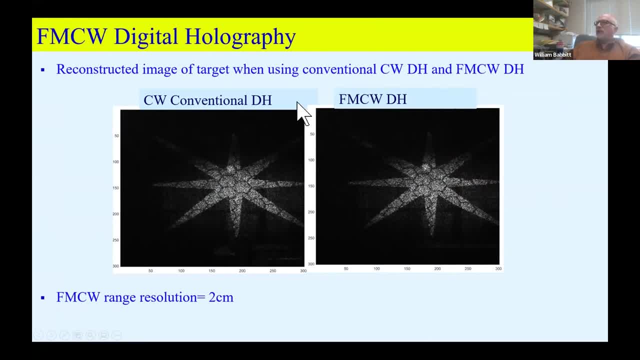 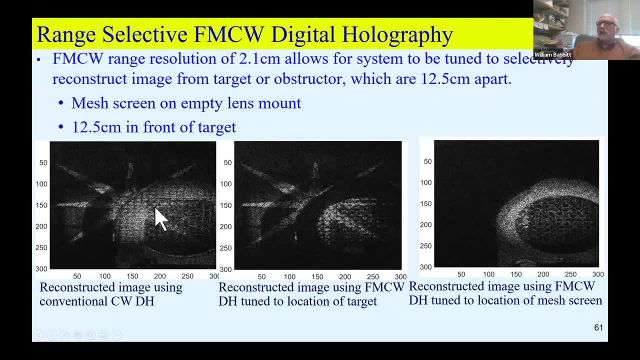 we really see very little difference between a CW conventional DH and our FMCW DH. But when we have a screen in front of it, here's the conventional digital holography. When we use FMCW, we can either focus on the star target. 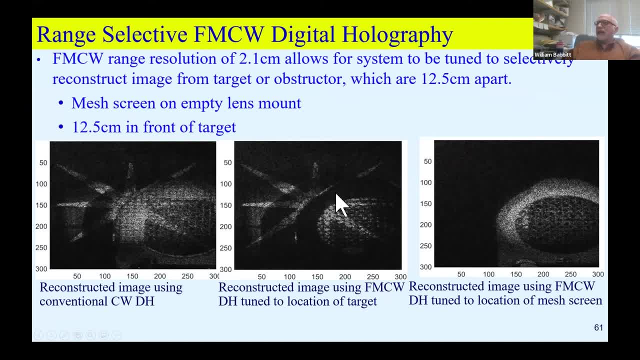 in which case we the here's the lens mounts blacked out, or we can change that frequency shift to look at just the scatter in front. So we can buy, we can actually have range selected digital holography, And these were about 12 centimeters apart. 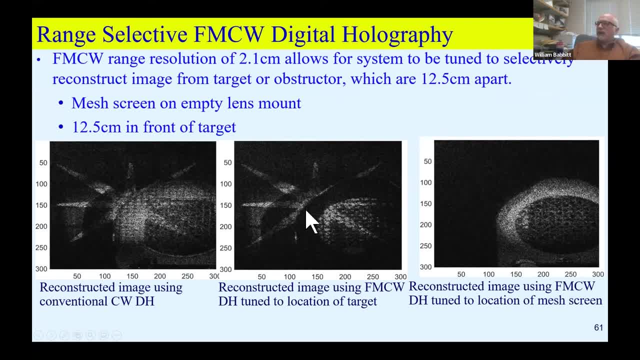 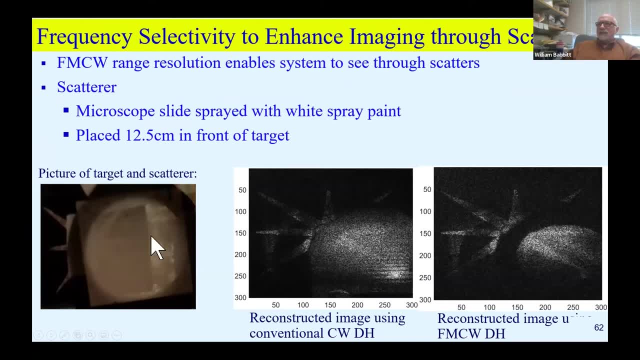 We have range activity here on the order of two centimeters, which a conventional holography you cannot get. The only interesting thing is that let's say you had a scatterer In front of your target And you. here's a picture of that. 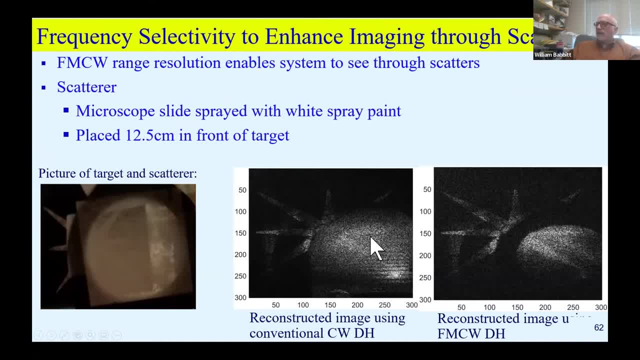 Here's the conventional CW DH And what we see is we can barely see the star pattern here. But with the FMCW, digital holography, we can actually pick out the star, return from the star and eliminate the scattering, And there you can actually almost. 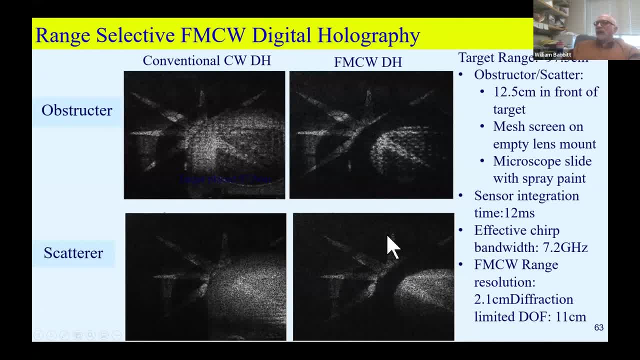 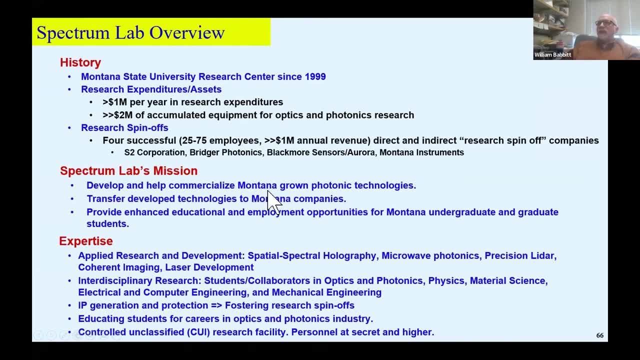 you can see through the scatter. Um I just a little bit about spectrum lab. We're part of Montana State University. about a million dollars a year. We help develop and help commercialize and grow companies. We're part of the university. 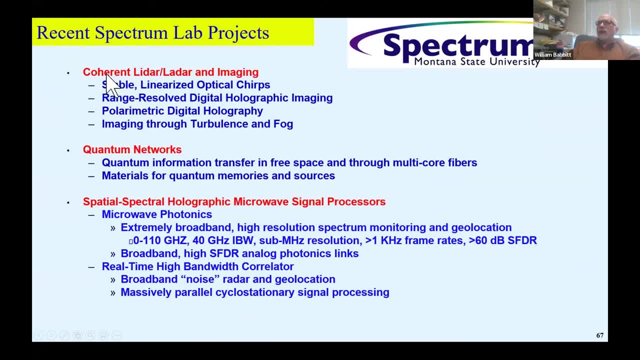 So we don't. we're not commercial ourselves. We work on both this coherent lidar and imaging, on networks, And some of the past work we've done has been on spatial spectral holographic microwave signal processors. Montana has on the order of 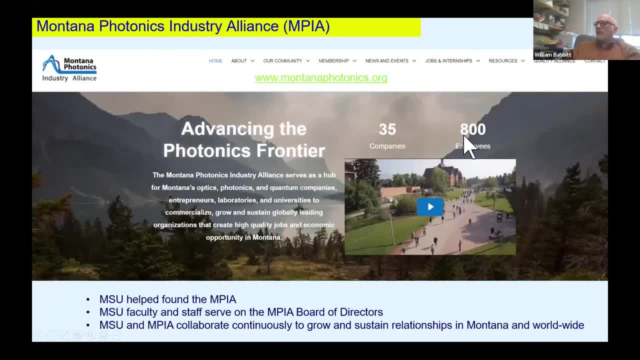 35 optics companies in Bozeman with I think it's over a thousand employees now, And so we kind of like to think of Bozeman or the Gallatin Valley as the photonic Valley in the US. We have the most optics companies per capita. 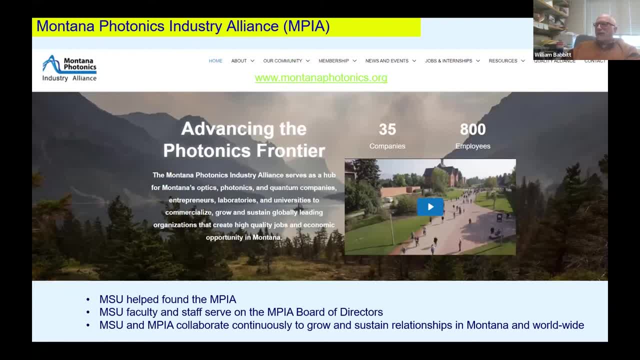 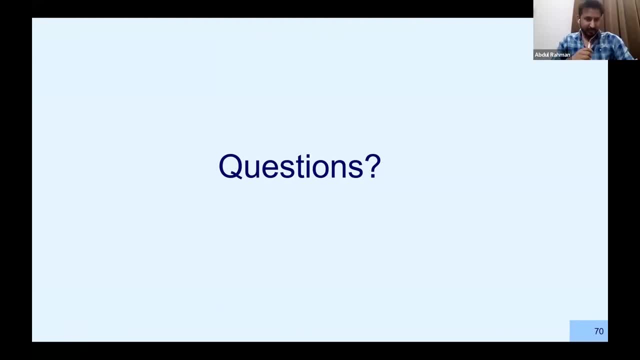 but we don't have many people. So when you divide by zero you get a big number. So that's my talk. Any questions? Okay, Thank you so much, Randall, for this wonderful, informative talk. So for the participants. 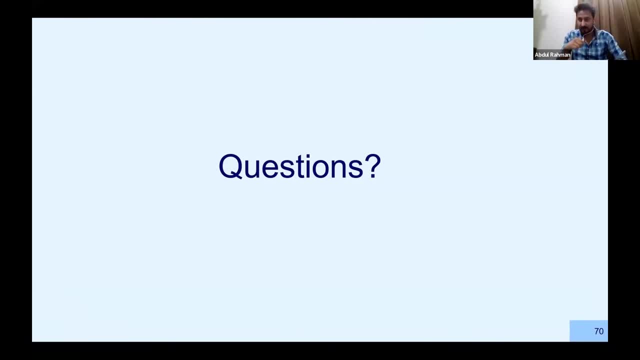 anyone who wants to ask question, please raise your hand. Okay, I think there is one question from Shehzad Ali. Okay, Shehzad Ali, you can unmute and ask your question please. I'm not hearing anything, Okay. 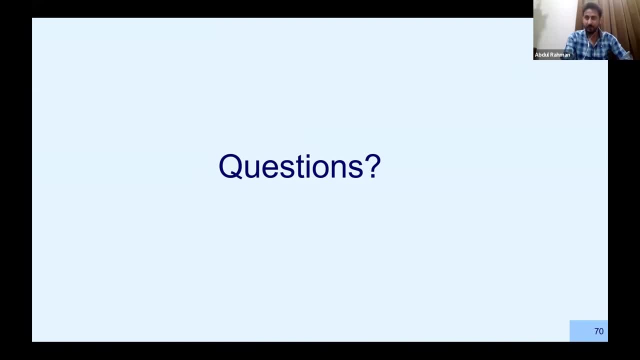 Okay, Then the next question is from Liru. okay, Liru, you can go ahead. Hello, Thank you for your presentation. It's very interesting And I have some questions. The first one is: how could we analyze the noise? 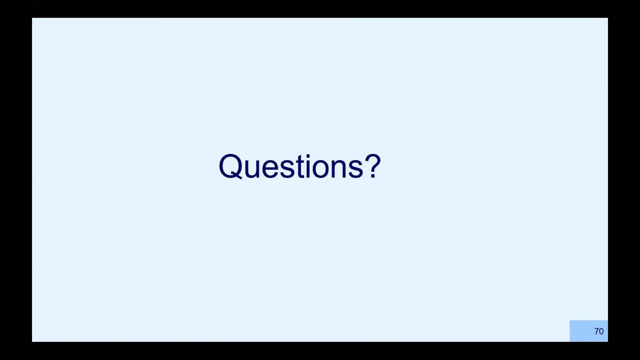 I think in the data there are many noise. How could we analyze noise? How can we analyze and analyze the noise accuracy? Thank you, How can you analyze the noise accuracy? Yes, What is the noise accuracy? How do you configure? 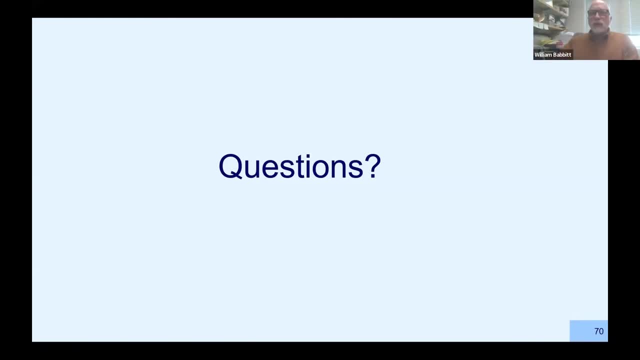 How do you, how do you measure the accuracy at which your system is working? Well, you have to have another way of calibrating your targets and knowing the the range distances between targets. So that's one way to characterize the accuracy. Is that what you're asking? 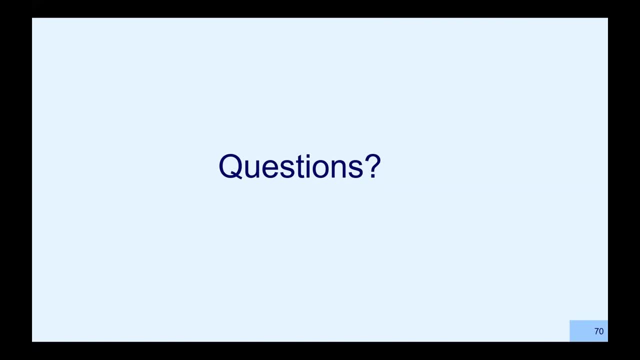 The accuracy of the system. Maybe in our world, how can we analyze the height accuracy? Because you see, in the LiDAR layer- many, I think in LiDAR, in one place- there are many different point clouds. So how can we analyze which point clouds choose the real height? 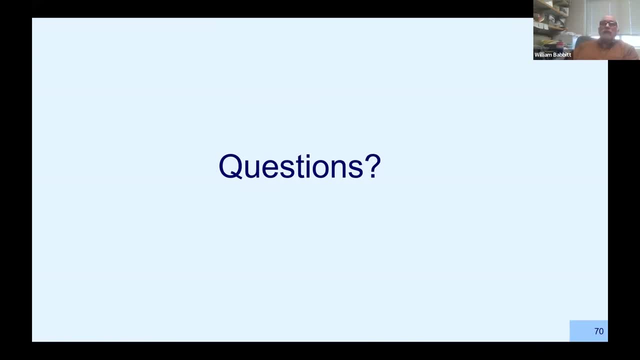 The only way to really do that is either compare multiple point clouds with one another and compare them, or use some sort of a reference to measure that. I think that's the only really way to measure the accuracy at which it's going. The accuracy is dependent on your chirp rate. 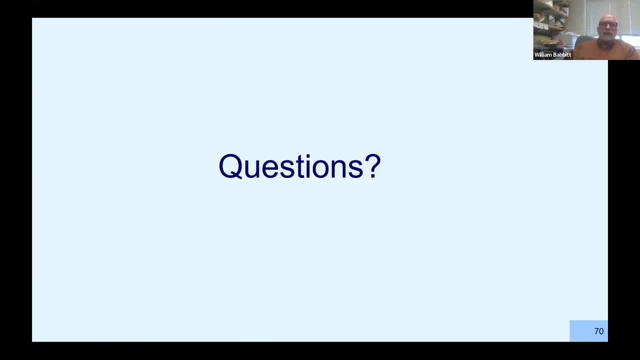 And so you need a very, you need a very accurate chirp rate, and that's usually done by comparing it to a reference or producing it digitally. Okay, Okay, Okay, Thank you. Thank you for your opinion. Thank you, You're welcome. 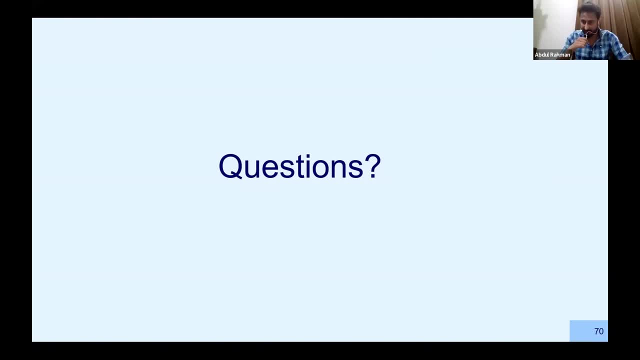 Any other question from the participant. Please raise your hand. We still have one or two minutes, maybe. Well, while people are waiting to raise their hand, Randy, So Tom Mossberg was your advisor. Yeah, he was my graduate advisor. 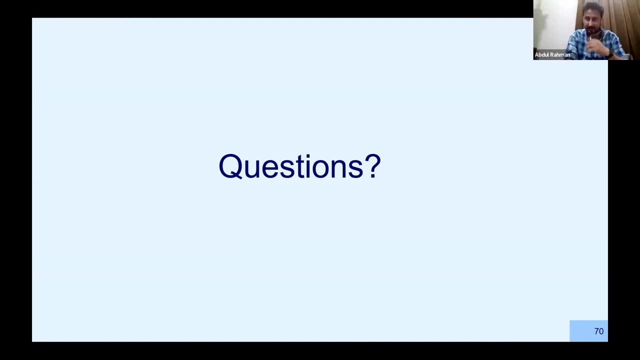 Yes, Really, Okay, Sorry, Oh, okay, Now we have a question. Yeah, She's oddly, you can ask now, And my question is: what is the distance distribution of random point in a cluster environment? What is the distribution? 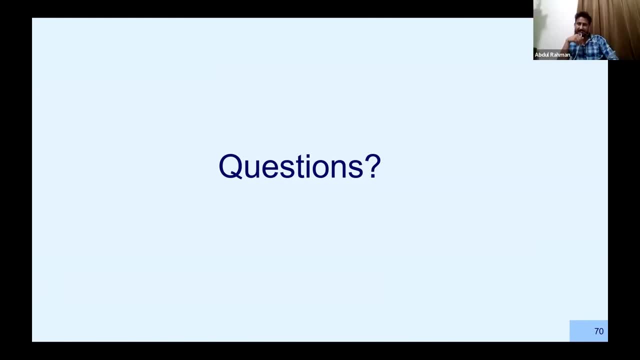 I'd say that again, please. She's oddly. can you please repeat your question? What is that distance distribution of random point in a cluster environment? Ran and I didn't quite. it's the, the, the, the, the transmissions being garbled. Can you say that one more time? 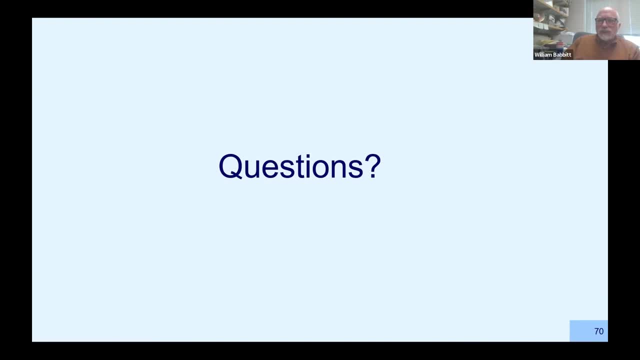 The random I got distribution of something She has odd. Can you please say it slowly, because it's a bit noisy from your side or maybe from the system. Okay, what? what is the distance Distribution of random point in our crystal environment? 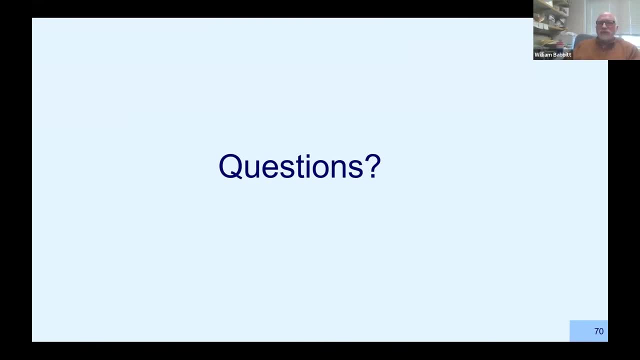 Oh, what is the? what is the distance, the distribution of distances and the and the targets we were looking at? Well, one of those- it was actually San Francisco, So it was an entire street of the point cloud was over by half a kilometer or so. 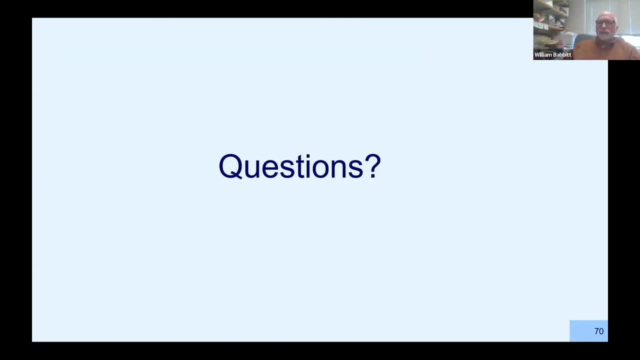 We and our measurements. that we were doing were tabletop measurements, were on the order of a meter distance, But they've done full several kilometer measurements as well. So it can. it depends on how long you're willing to wait the for the scan And 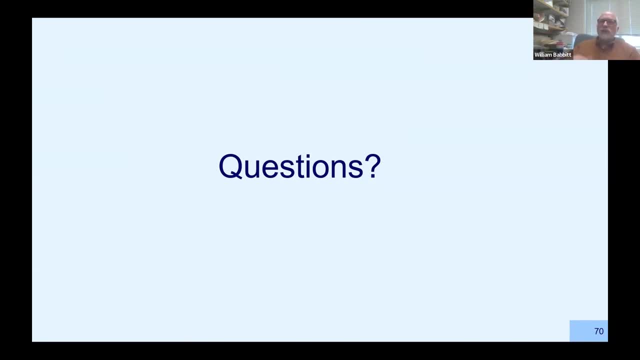 and integrate points is how large a distribution of point clouds, how long a larger point cloud you can do. Does that answer your question? She's odd. Did you get your answer? You'll be Okay. I think the network from his side is a bit noisy. 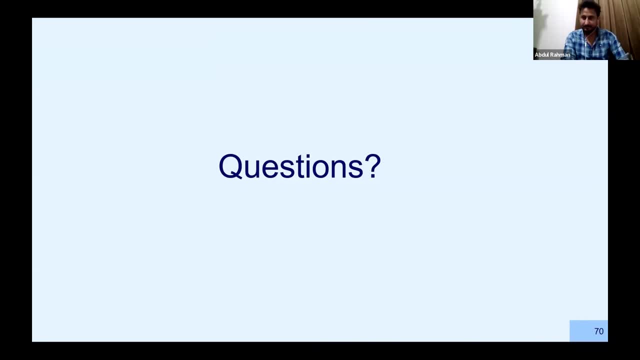 So any other question from the participant? Yeah, I got you though. Yeah, okay, Yeah, you go, you can unmute and ask, please. Thank you very much for this presentation, Very informative. I have a quick question. I've tried making a. it's an open source.